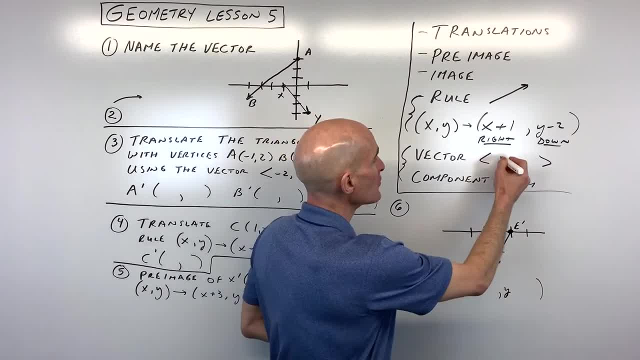 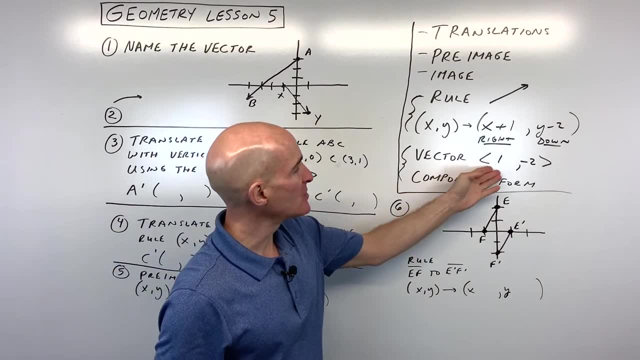 it does is we can do the same thing using a rule, using a vector. We can say one negative two. Now notice, these aren't parentheses, They're more like these triangular brackets, And what this represents again is just: we're going to be adding one to the x coordinates, We're going to 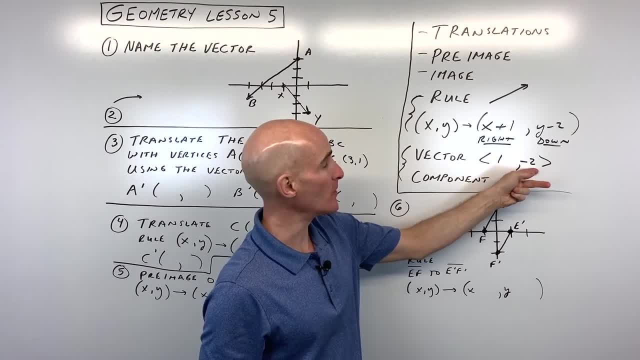 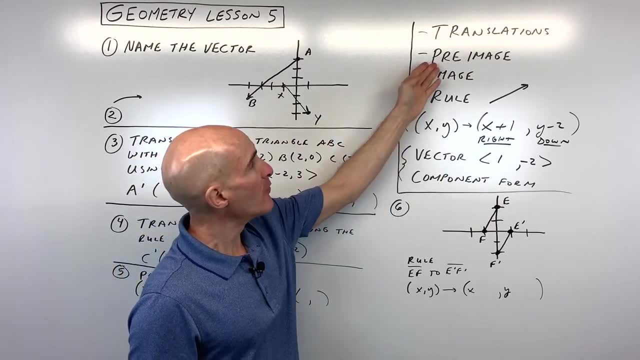 be subtracting two from the y coordinates. It's going to shift the y coordinates. We're going to shift right one, down two. So two different ways, using a rule or a vector to do a translation. That's what we're going to be talking about first. Another thing: we want to talk about some other. 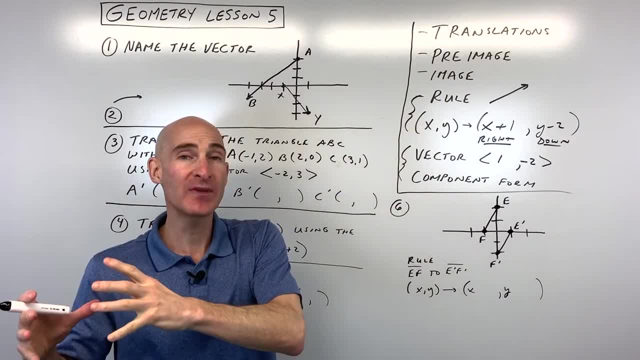 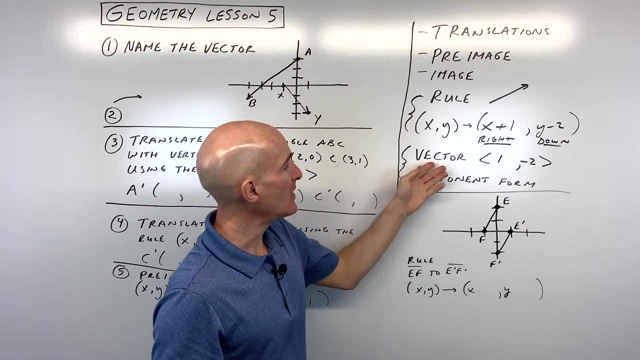 definitions: pre-image and image. Pre-image means before And then image means after. you've done that translation, okay. So pre, just think before, Pre-image, and image after. And then again we talked about our vector component form. Let's jump into some examples. The first one: what we want to. 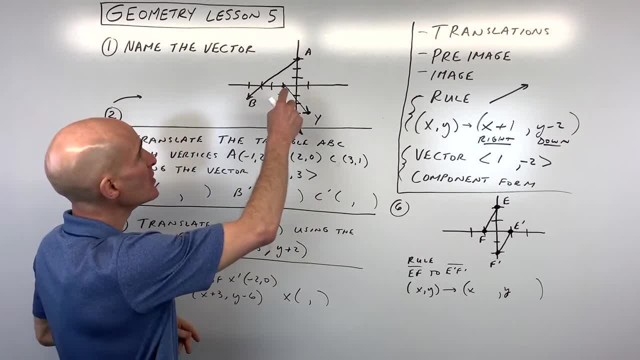 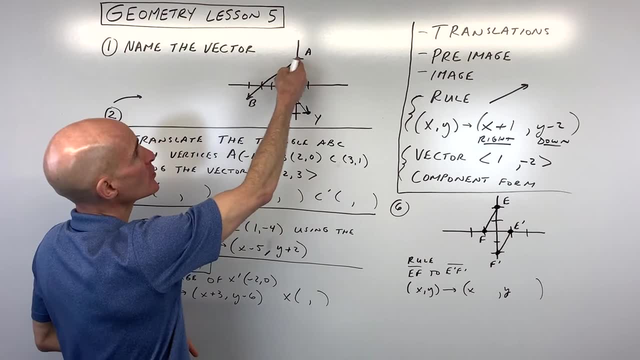 do is talk about how do you actually name a vector. So here, let's say I was going from point A to point B. They call this the initial point, They call this the terminal point. So we're going from A towards B, here 2B, And to get there, you can see I'm going to have to go. let's see left. 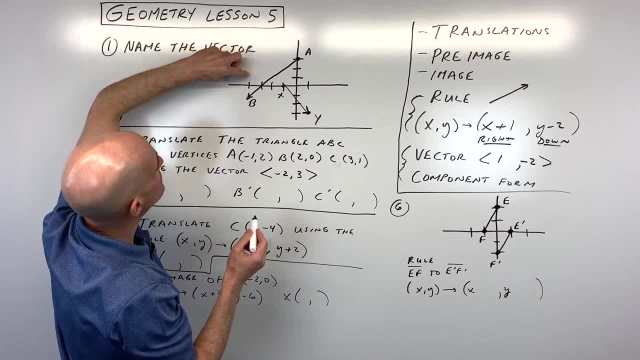 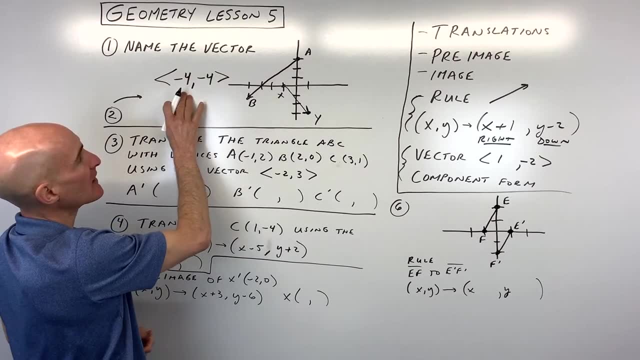 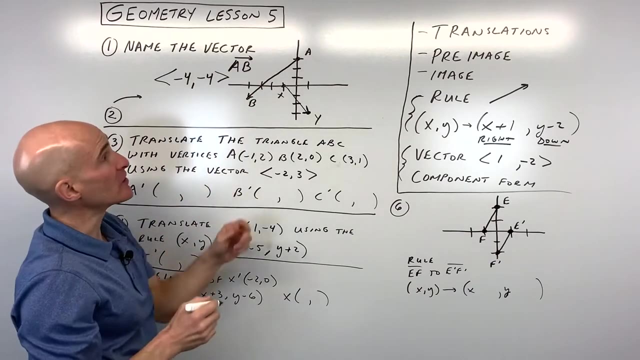 one, two, three, four and then down one, two, three, four. So we can write this in component form: negative four, negative four. Okay, that's left four, down four. But the way we would name it it's going from A to B, like so Let's look at another example, See how you would do this one. 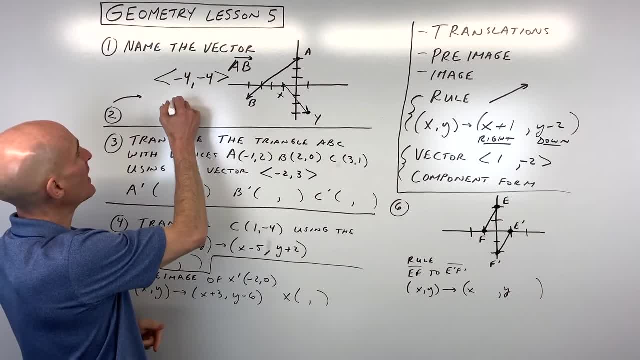 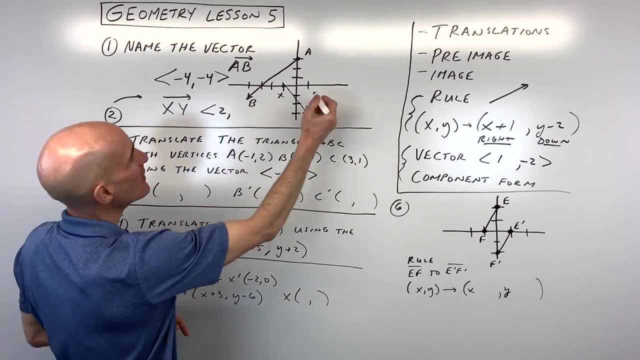 vector XY. Okay, so if we name it it's just vector XY, like that from X to Y, And you can see, here we're going right two, So that's going to be positive two, And then we're going down. 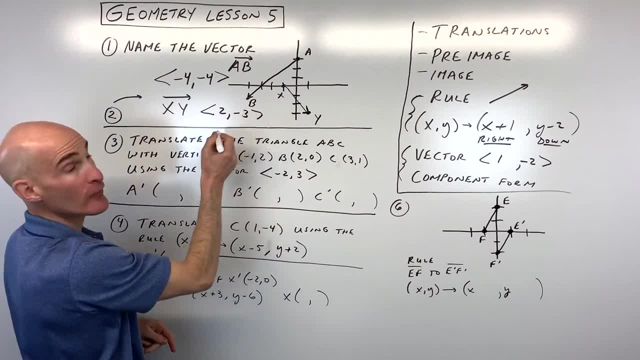 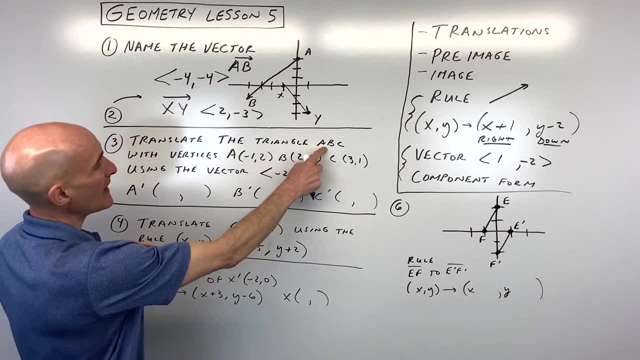 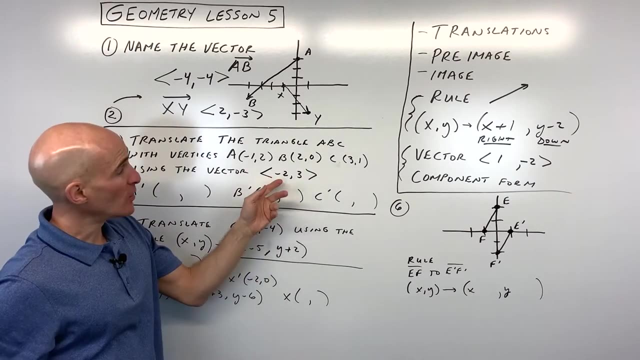 three, That's negative three. So that's our component form of our vector XY: two negative three. Let's jump into number three now. It says: translate the triangle ABC with vertices A, B and C using the vector negative two, three. So what this vector does is it shifts, it left two. 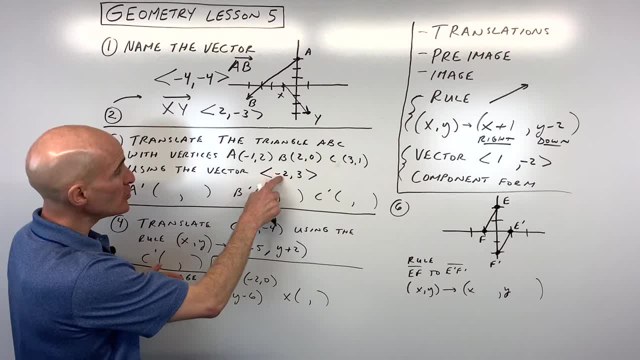 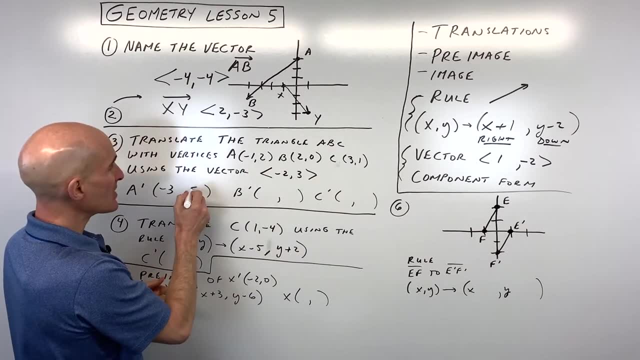 and up three, the triangle. And what you can do is you can subtract two from the X coordinates, So negative one minus two is going to be negative three, And add three to the Y coordinates, So that's going to put us at five For B prime. this is a new coordinate of B. Two minus two is going. 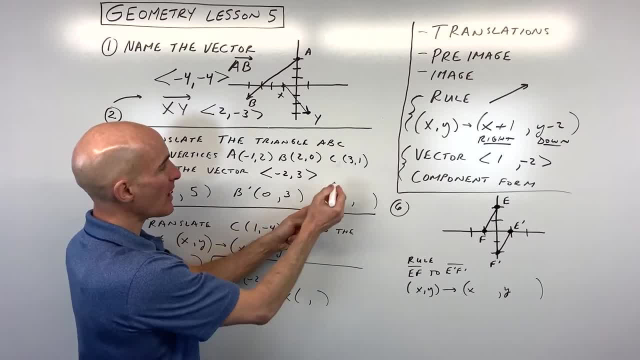 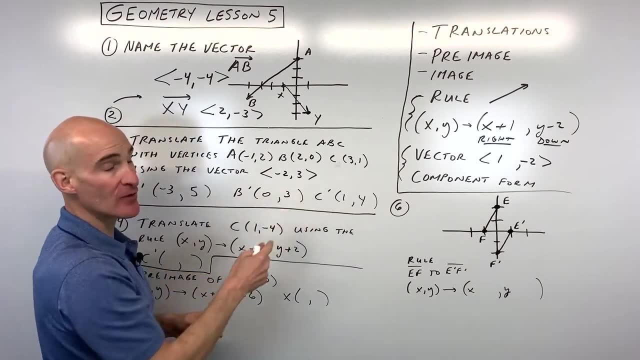 to give us zero, And zero plus three gives us three, And then C prime we have three plus negative two is one, And one plus three is zero, And then C prime we have three plus negative two is one. Notice that the prime, this little apostrophe here, represents the image, the new coordinates of 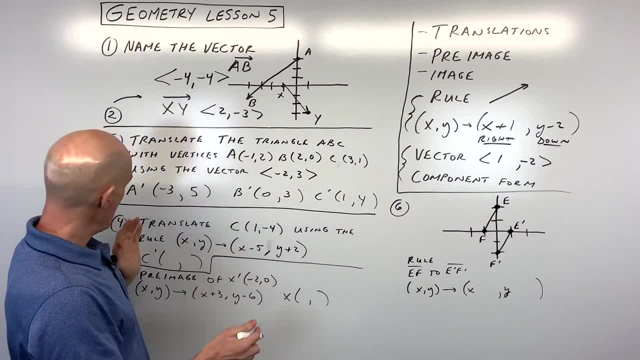 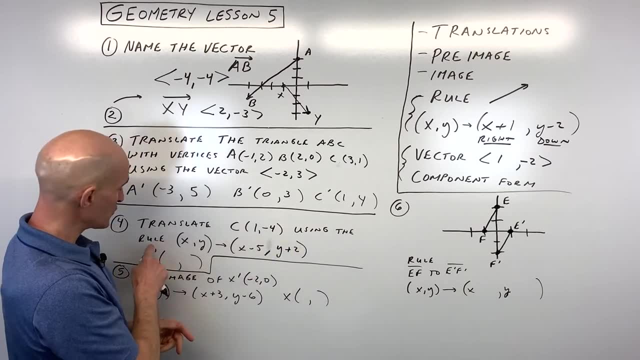 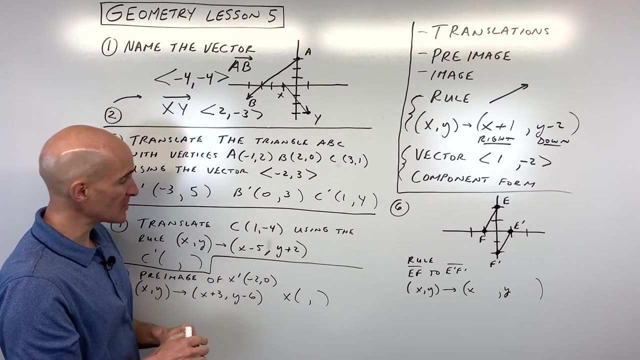 the point, whereas the ones without the prime. that's the pre-image. Okay, for number four. what we're doing here is we're translating the points C, one comma negative four, using this rule: XY maps to X minus five, Y plus two And C prime. our new coordinate for point C is going: 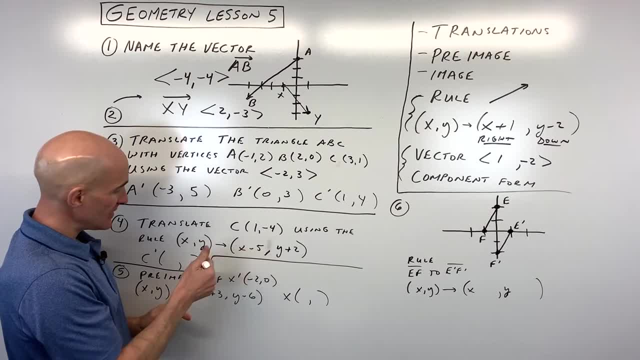 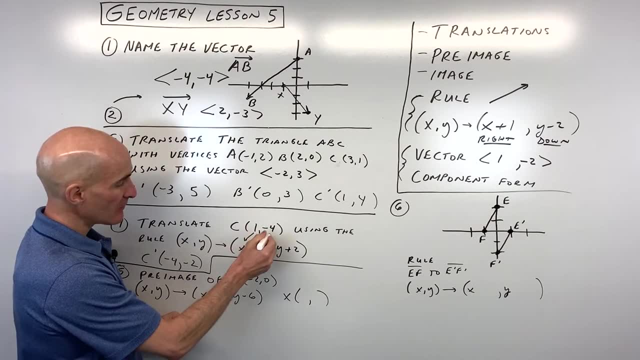 to be what. Well, you can see, one minus five is negative four, And C prime, our new coordinate for point C, is negative four plus two is negative two. So it's pretty easy. You're substituting in the X for X, Y for Y. This just says we're going left five and then up two And you've got your. 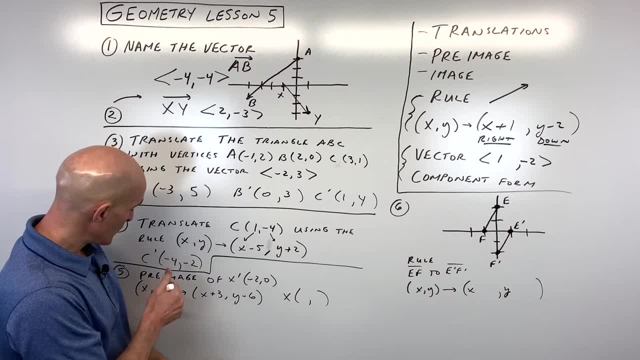 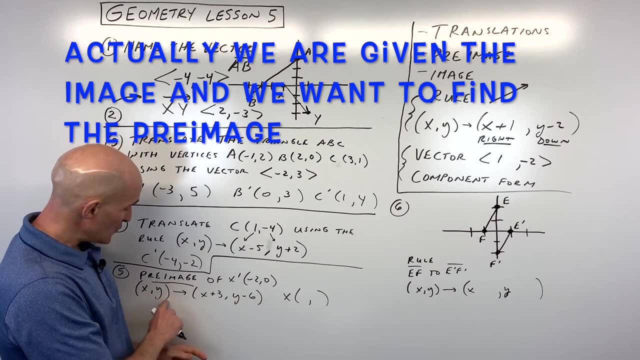 new point For number five. this one's a little bit more challenging because what they're doing is they're giving us the pre-image. They're saying X prime. this point, X prime negative two zero is being translated using this rule: X plus three, Y minus six. So how do we get back to the original? 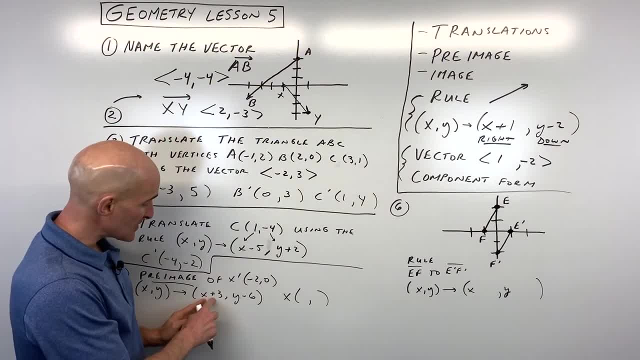 point before the translation. Well, we're going to have to do the opposite: Instead of adding three, we're going to have to subtract three from negative two, which puts us at negative five. Instead of subtracting six, we're going to have to do the opposite of subtracting: We're going to 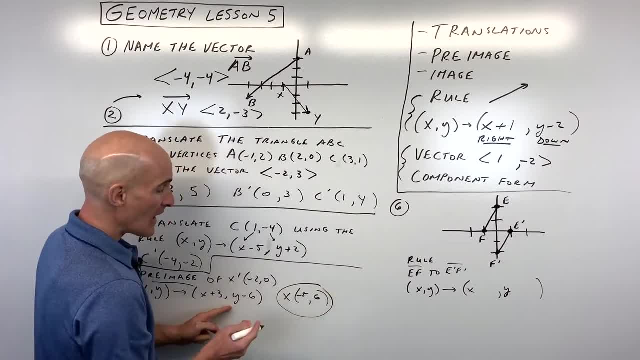 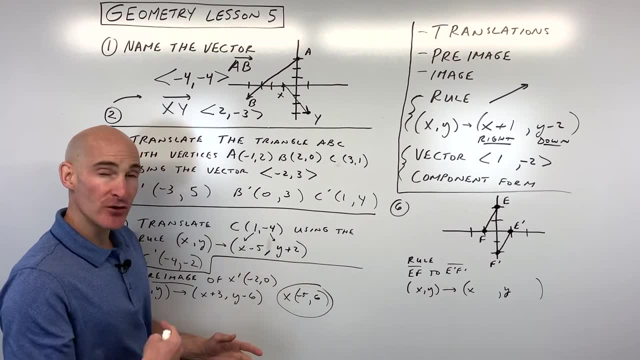 have to add six. So zero plus six is six. And again you can check your work. If you take negative five plus three, that gives us negative two and six minus six is zero. So we had to reverse it and adding and subtracting our inverses or opposites. So if you just do the opposite you'll get the 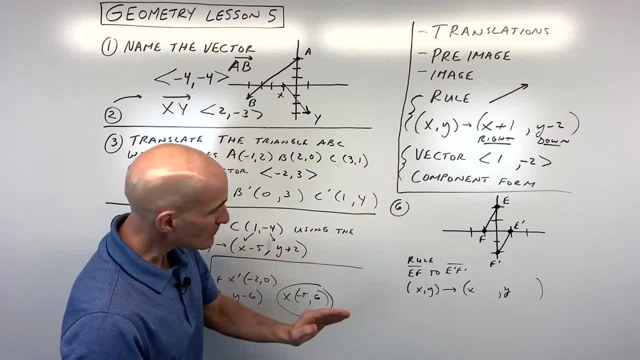 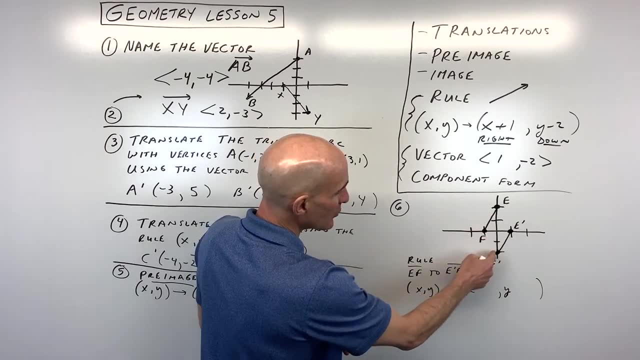 original point. And then for number six: here, what we want to do is we want to come up with our own rule that translates This segment, EF, to this new segment here: E, prime, F, prime- And you can see that it's actually like: 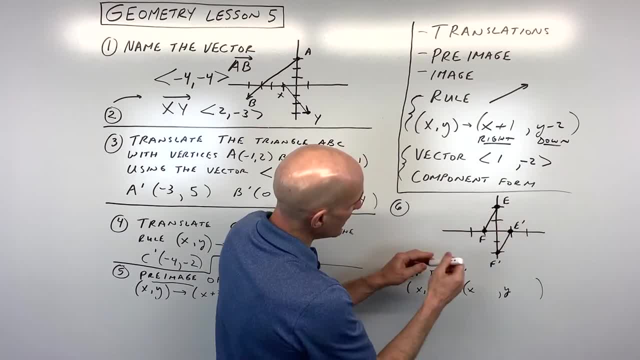 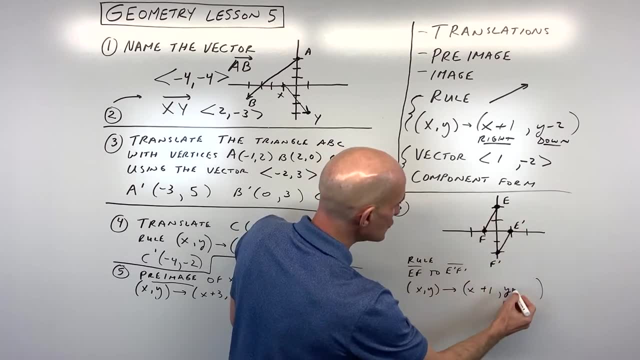 we're picking up this segment, We're shifting it right so many and down so many. It looks like we're shifting right a one, So this would be like X plus one, And then we're going down two, So that would be negative two, So that would be a rule. If you wanted to write it as a vector, you could. 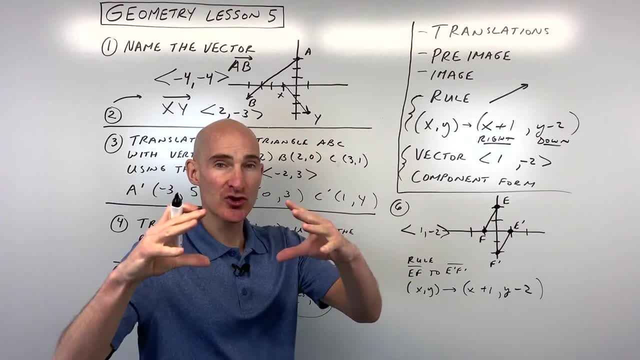 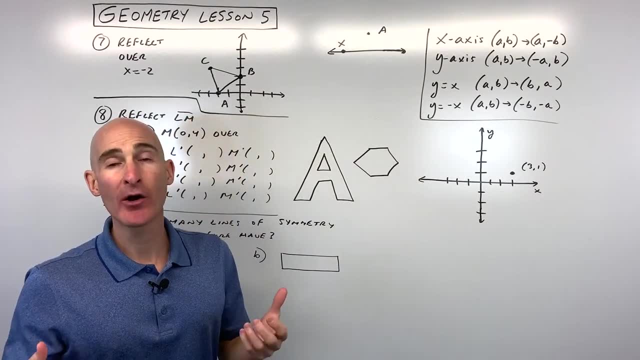 just say one comma negative two, And again make sure to use those triangular brackets to indicate that it's a vector. Let's talk about reflections. Okay, the next type of transformation we want to talk about are reflections. And what exactly is a? 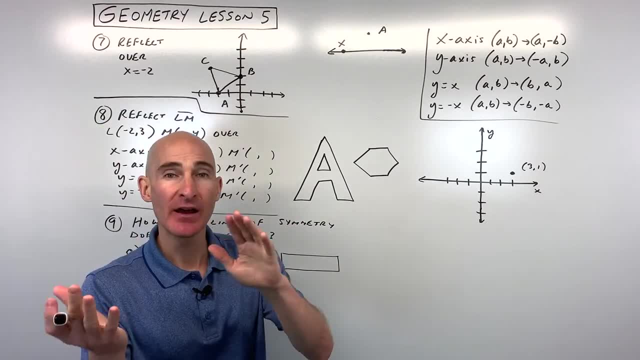 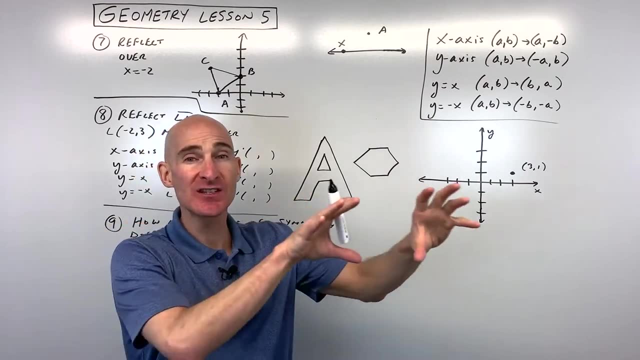 reflection. Well, a reflection is basically like a fold, Like, say, if you were to take something and like fold it over, you know kind of like flip it. That's what a reflection is. So a translation is a slide. a reflection is like a flip, And what we want to do is say, for example, we wanted to take 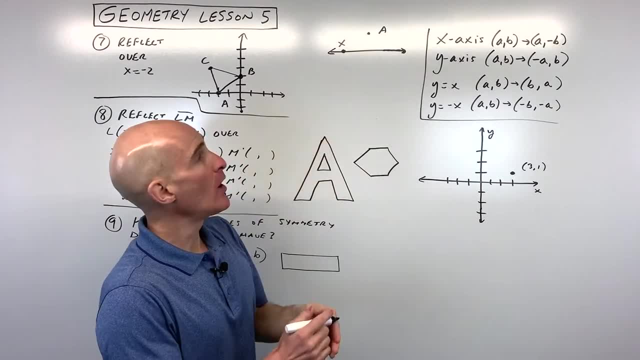 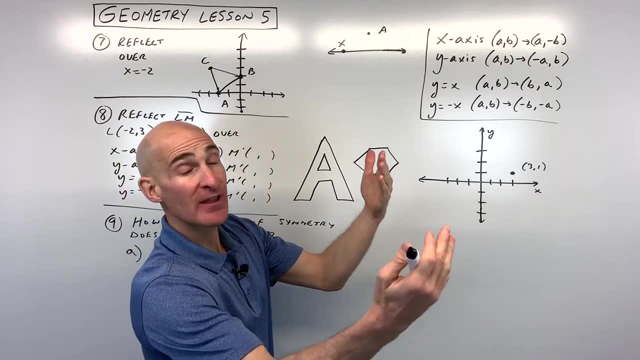 this point A and reflect it over this line. Well, it's just like when you look in a mirror, like if you look in a mirror and you're standing, let's say, a foot in front of the mirror and you're looking in the mirror, it looks like your reflection is a foot behind the mirror, right, And what you? 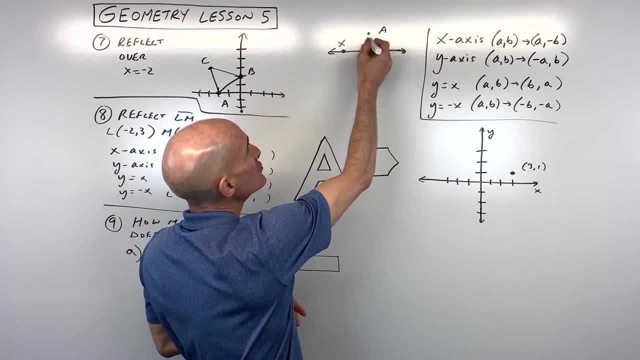 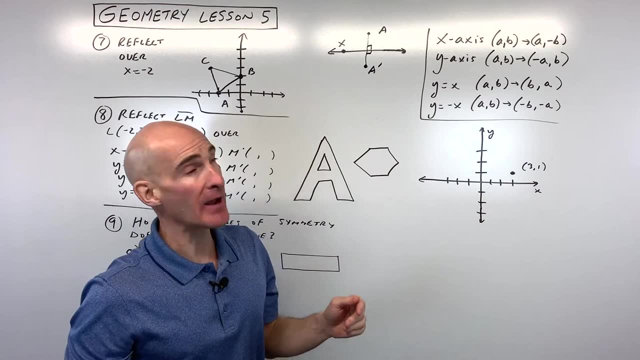 want to do is you want to find that perpendicular distance to that line of reflection. You want to go the same distance on the other side, and that's where your image is going to be A prime. Now, what happens if you put your nose right up against the mirror, right that line of reflection like axes? 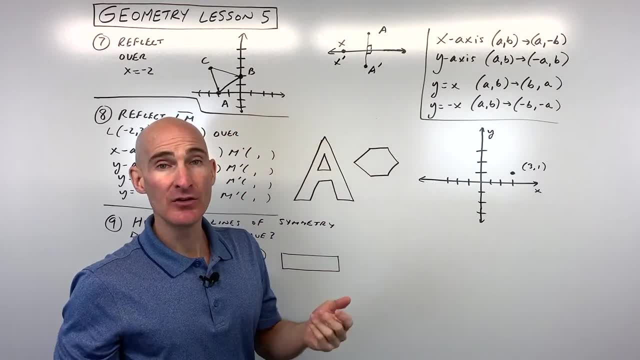 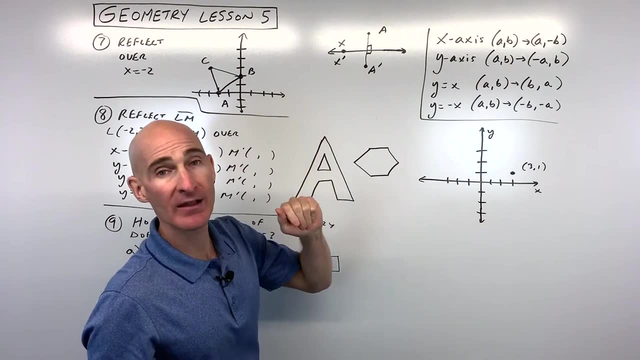 here. Well then, the image. okay, the new point is also going to be on that line of reflection, So it looks like your nose is touching from either side, if you put it right on that line of reflection. Now, what we're going to do is talk about reflections in the coordinate plane here. 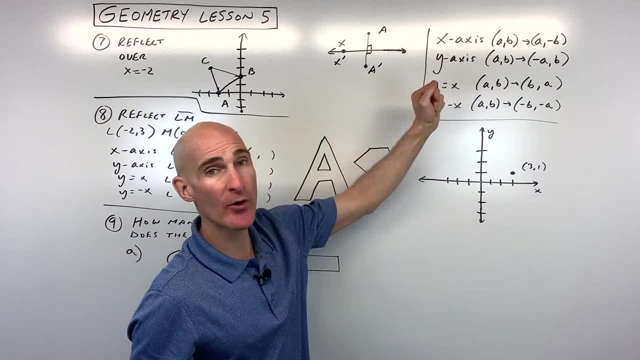 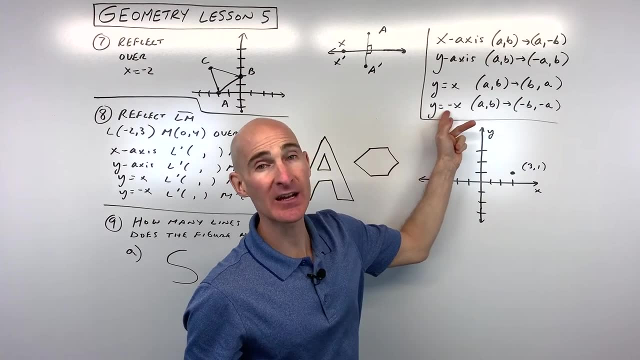 the xy plane and we've got some rules here that you might want to write down or memorize. If you're reflecting over the x-axis, y-axis, line y equals x and line y equals negative x. Now I want to show you just real quickly how to figure these out, in case you forget these formulas. 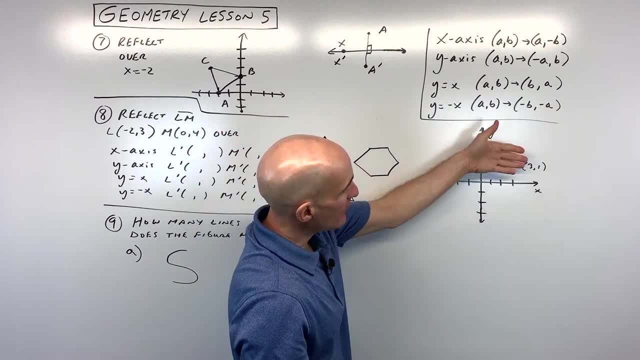 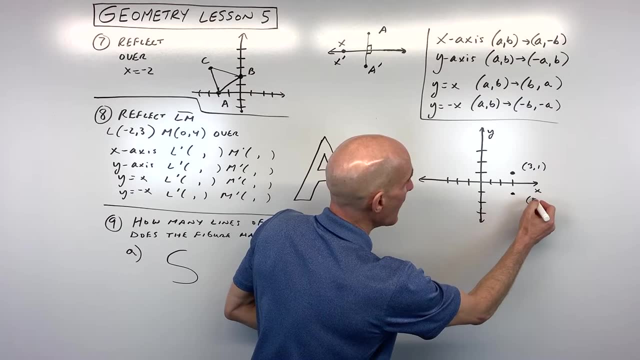 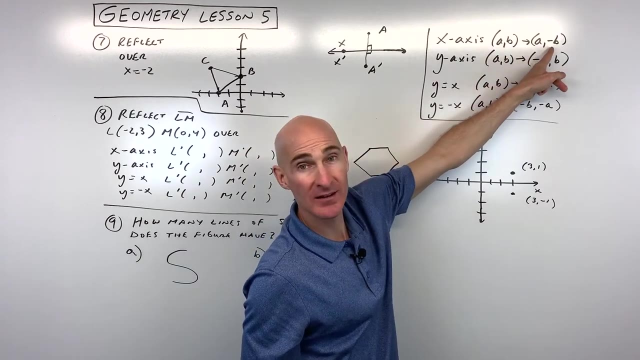 Let's take a point like the point. If I reflect it, okay, like, fold it over the x-axis. here you can see this point is going to end up right here at three comma negative one. So what happened when I reflected over the x-axis, It was the y-coordinate that became the 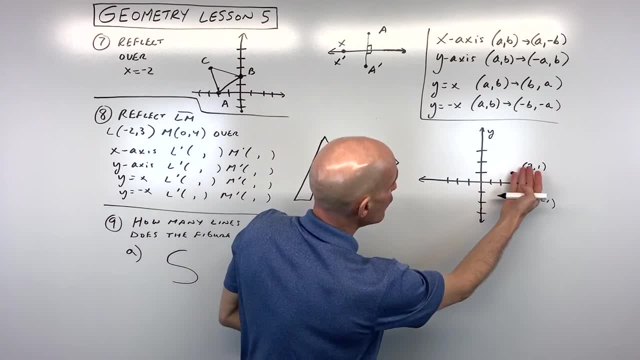 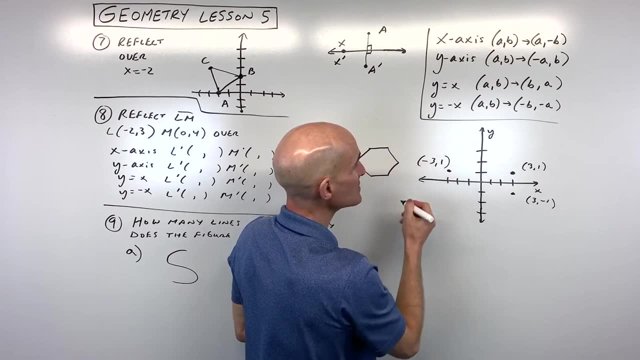 opposite. The x-coordinate stayed the same. If I reflect it over the y-axis, what happens? You can see if we fold it over this line here, it's going to be negative three, positive one. What happened here? It was the x-coordinate that became the opposite. The y stayed the same. When we reflect, 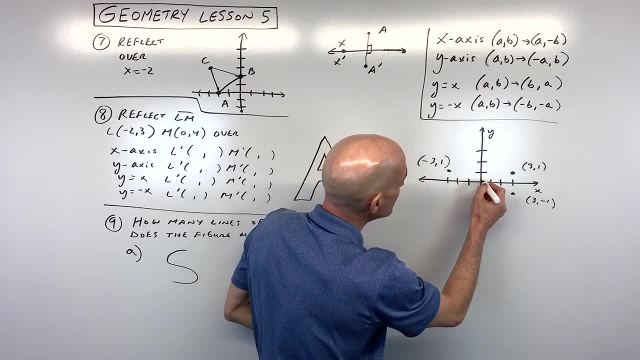 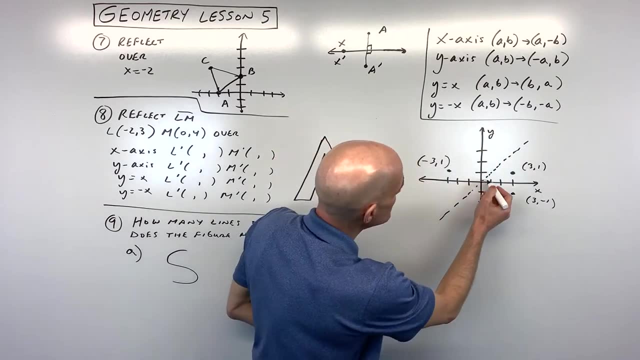 over the line y equals x. okay, this is a line with a slope, one that goes to the origin. Okay, so that's going to look something like this: a 45 degree line. If we fold it over that line, you can see that's going to put us right about there. Okay, if I've drawn my drawing, well. 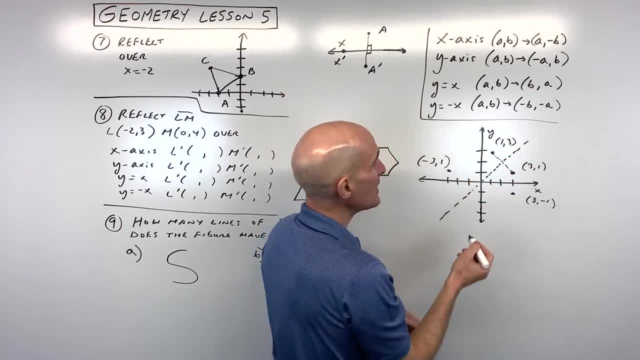 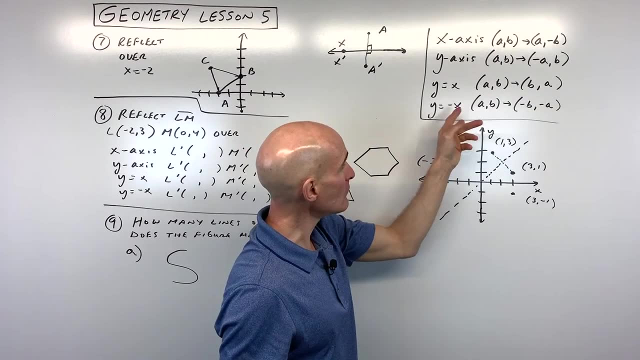 that point is actually going to be. the point- And you can see what happened here- is we actually interchange the x and y-coordinates. Instead of ab, we have ba, And then, if we reflect over the line, y equals negative x, that's a line that has a. 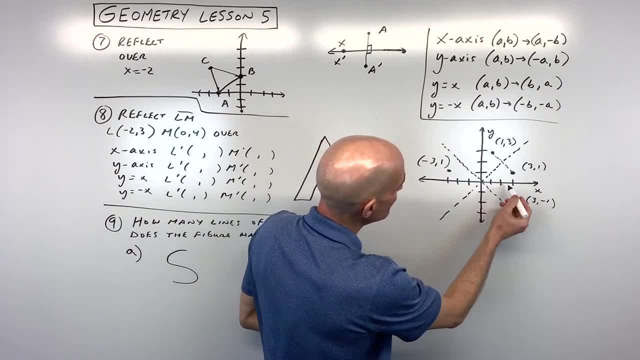 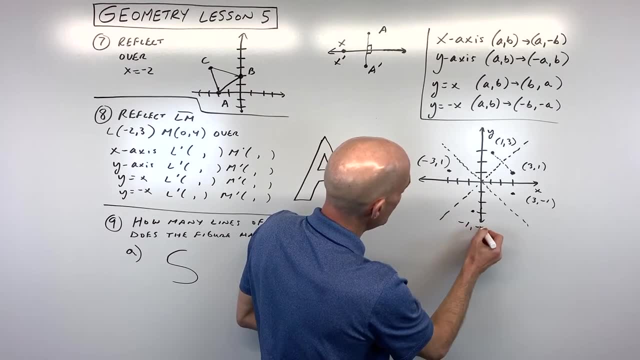 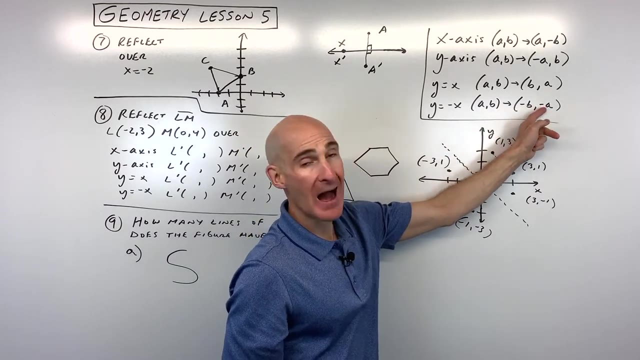 negative one slope okay and goes to the origin And if we reflect this point, it's actually going to go right here at negative one. negative three: See, I'm folding over that line And notice what happened here. We switched the x and y-coordinates and we made them the 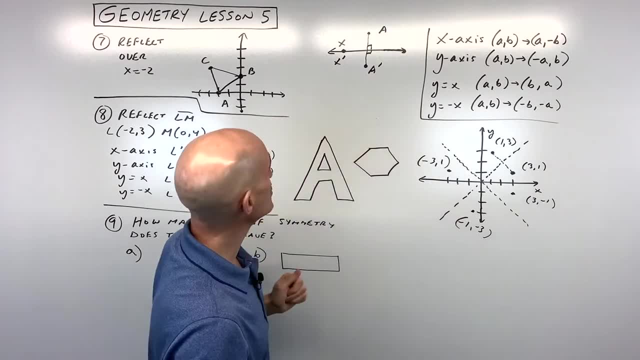 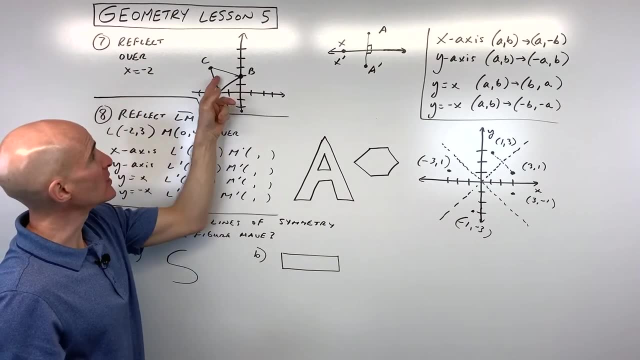 opposite signs. So these are the rules that we're going to use with reflections in the coordinate plane. Let's try some examples. Say, like number seven, we want to reflect over the line x equals negative two. We're going to take this triangle and reflect it over the. 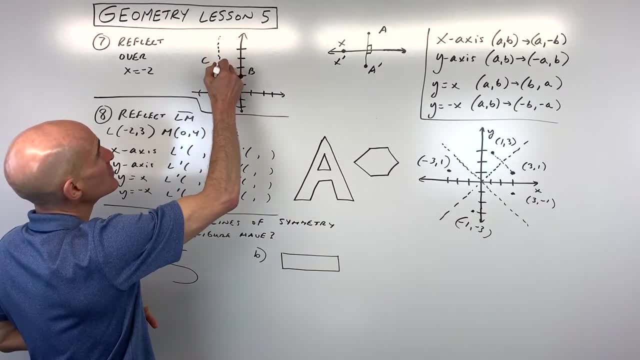 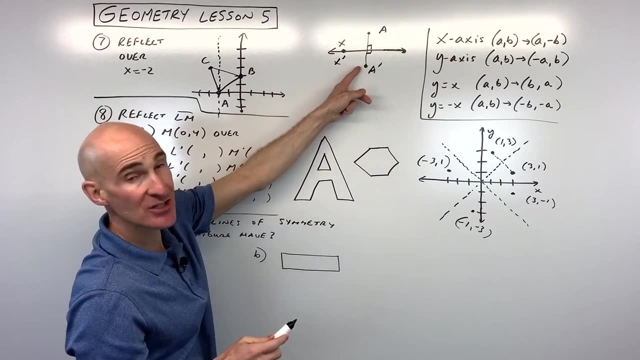 x equals negative two, which is a vertical line. Okay, x equals lines are vertical lines, And what we want to do is we want to fold it. Remember it's always the perpendicular distance to the line of reflection, the same distance on the other side. So here, a is right on that line. 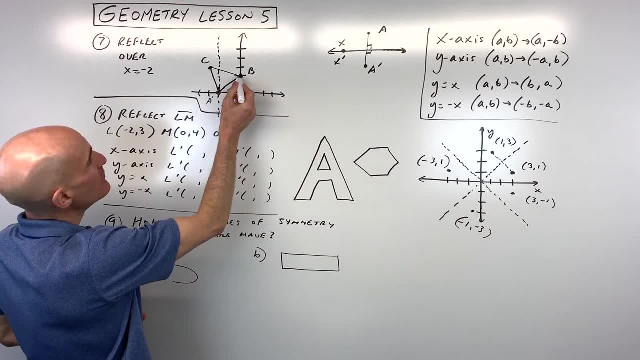 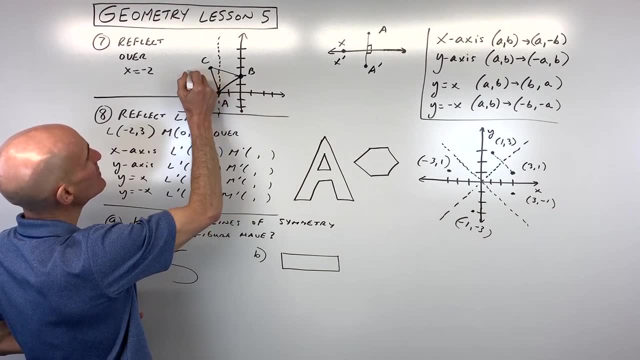 of reflection. So a prime is going to stay right there, B on the other hand, see how it's one, two units from the line of reflection. We're going to go one, two on the other side. So there's going to be b prime And then c is one to the left of the line of reflection. 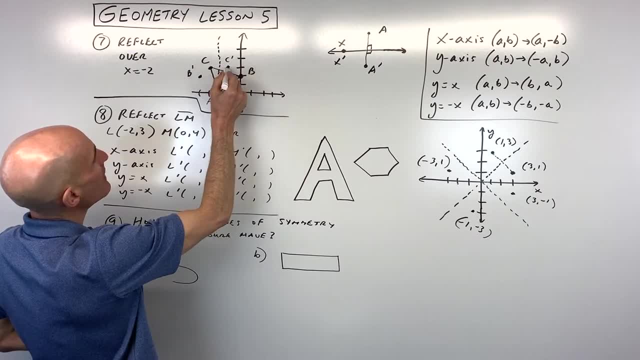 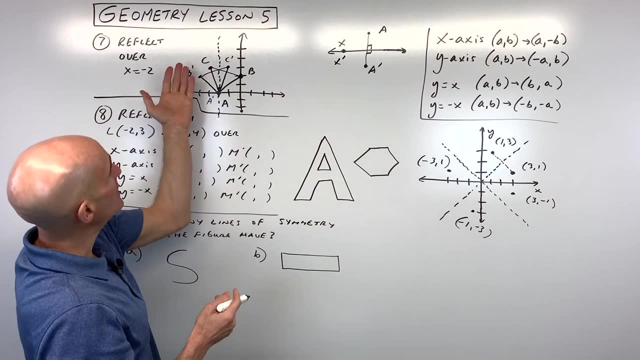 and we have to go one to the right at c prime. Now, if we connect those together, what does that look like here? Like that, So you can see if you've done it right. it should look very symmetrical. It should look like if we fold it, you know it's going to match. 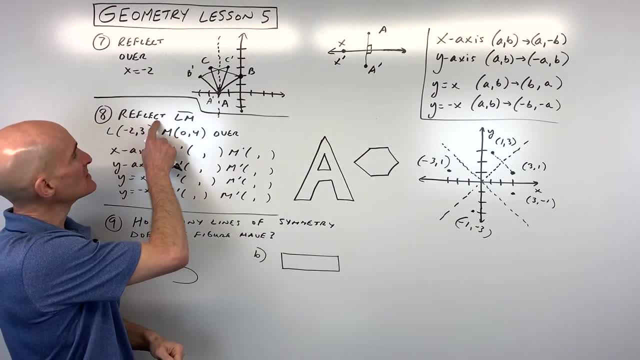 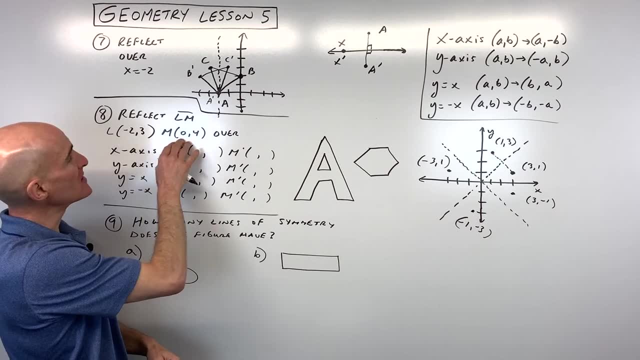 to itself. Let's look at number eight now. It says: take the segment l m, okay, and points l are negative. two, three, Point for m is zero, four, Those coordinates. We're going to take that line, segment l m, we're going to reflect it over the x-axis, y-axis, line y equals. 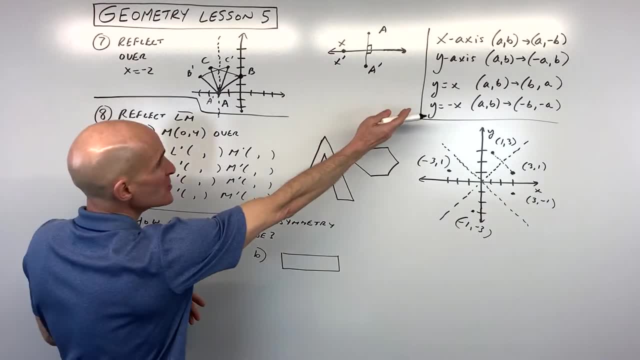 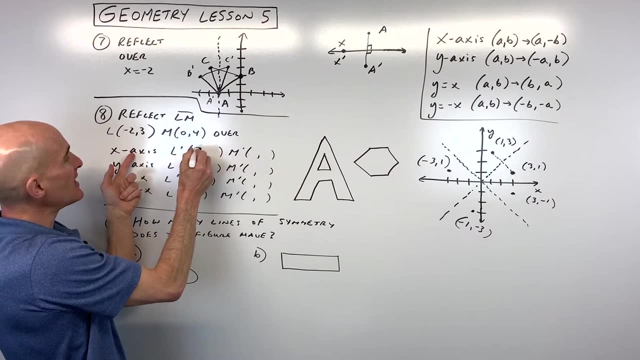 x and line y equals negative x. So what we're going to do is we're going to use these rules over here. Negative 2, 3.. If we reflect over the x-axis, the x stays the same right, but the y 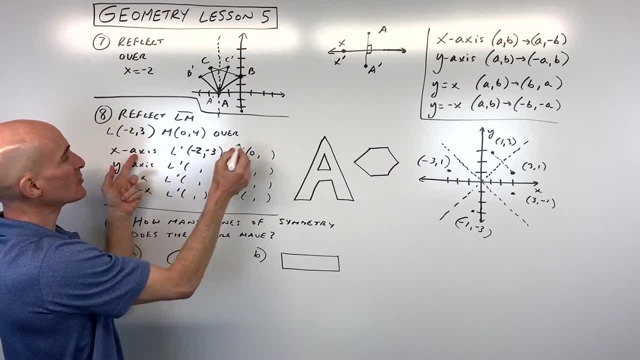 coordinate becomes the opposite sign. So this becomes negative 3,. this becomes negative 4.. If we reflect over the y-axis, the y-coordinate stays the same, but the x-coordinate becomes the opposite. Of course, the opposite of 0 is still 0, right? If we reflect over the line, y equals x. this: 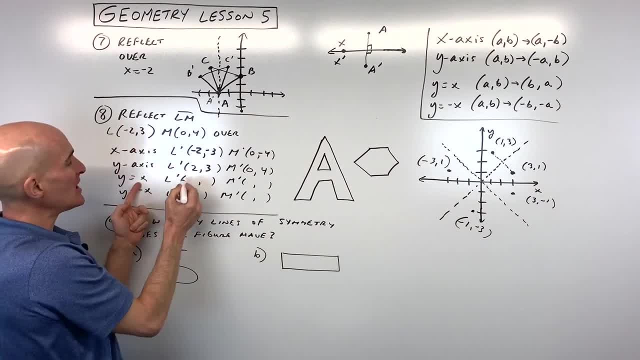 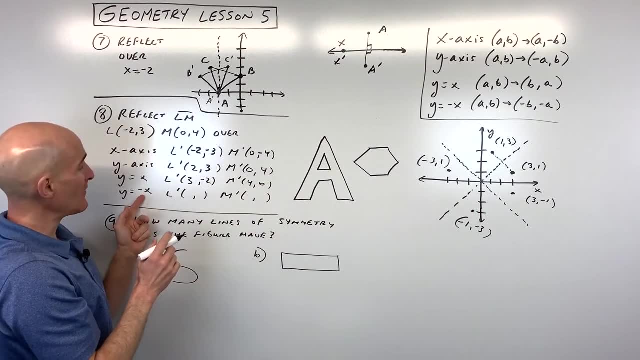 45 degree line. here what we do is we actually interchange the x and y coordinates. so we're just changing the order x and y, we flip, and when we reflect over the line, y equals negative x, we switch the order and we switch the sign. okay, so this becomes negative 4,. 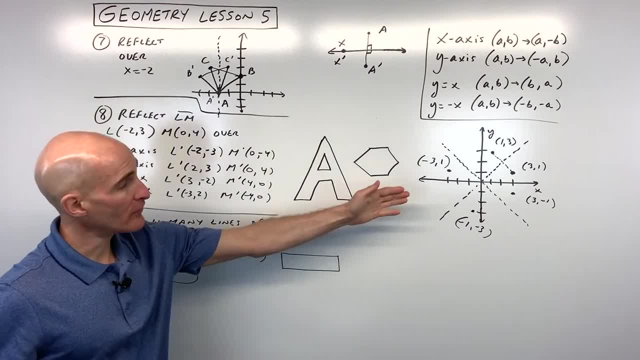 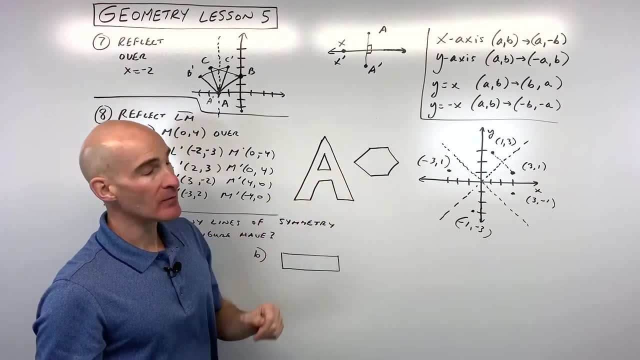 0, and you got it. so again, just knowing those rules is key, or, if you want, you can draw it out, and that'll help you as well. Now let's talk about lines of symmetry. now, when we look at some figures or polygons, 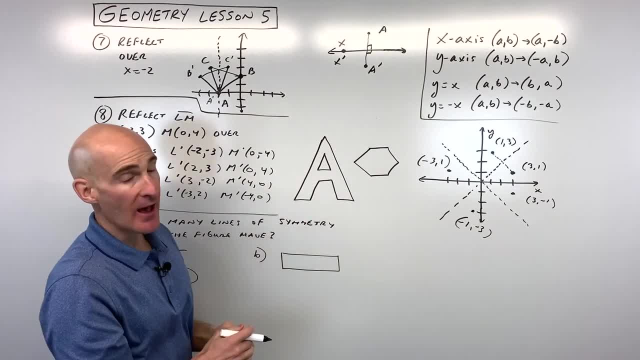 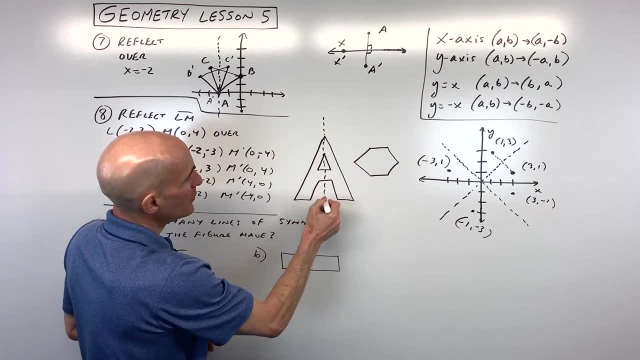 or objects. how many lines of symmetry does this letter A have meaning? how many ways can we fold it over that line so that it matches to itself? well, here you can see, it looks like there's only going to be one. if I fold it this way, it's going to match to itself. 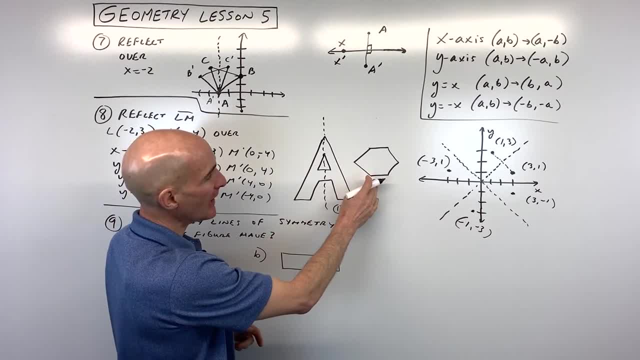 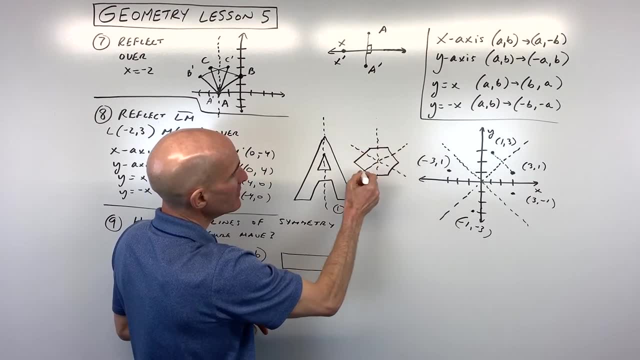 so it looks like there's only one line of reflection here for this hexagon. how many lines? it looks like we have one here, two there, three there. you can also go through the vertices like this: four, five, Six. okay, so if you fold over all those lines, it's going to match to itself. so this one. 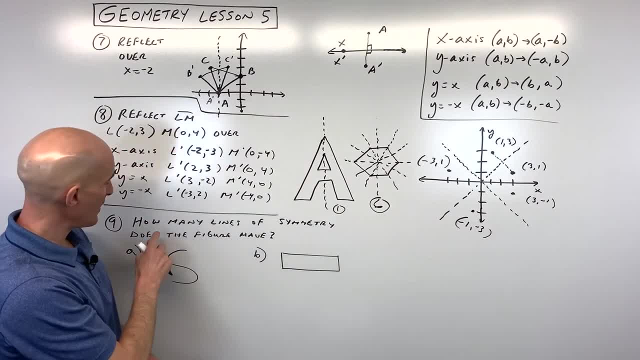 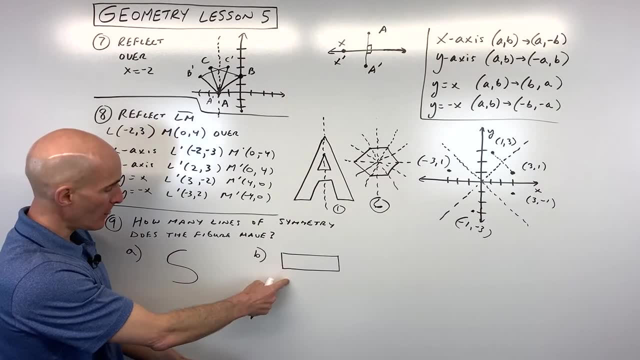 has six lines of symmetry. try these ones for number nine. how many lines of symmetry does the figure have? for letter A, it looks like the letter S. for letter B it's like a rectangle. Now for this one. when you look at the letter S, you might say to yourself: Mario can't. 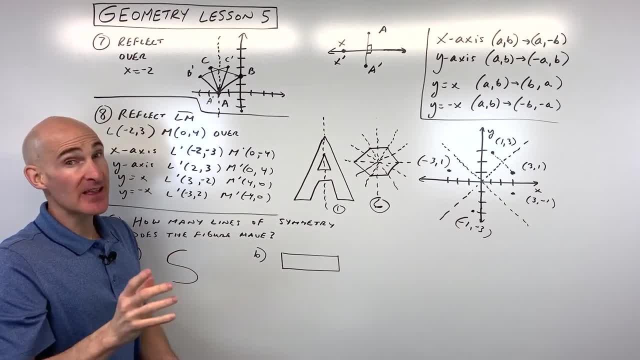 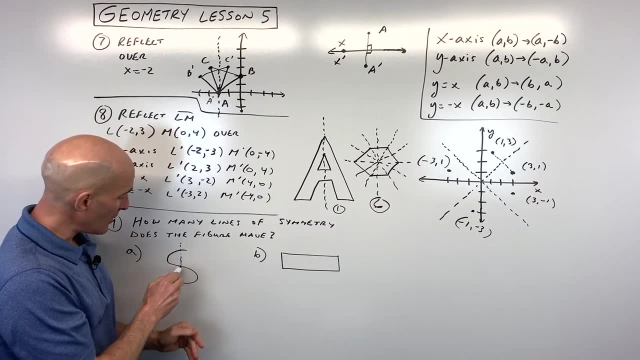 I just like pick this up and rotate it and it'll match to itself. yeah, that's a rotation and we're going to talk about that coming up here in just a couple minutes. but as far as lines of symmetry, If I try to draw a line like this, okay, if I reflect this over here, that doesn't match. 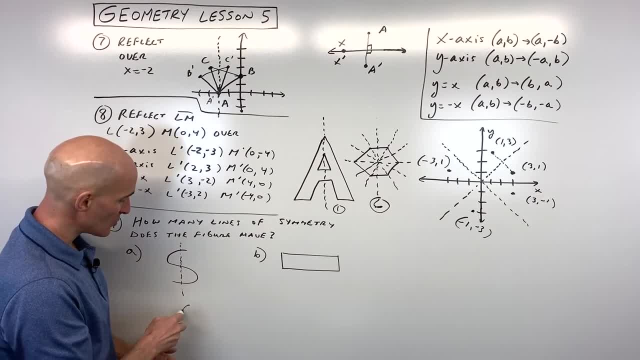 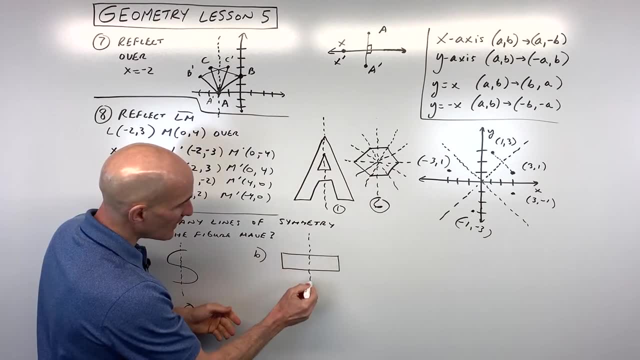 up. if I reflect this over here, it doesn't match up. so this one actually has zero lines of symmetry For letter B. what do you think for this one? any lines of symmetry here? well, you can see, definitely, going right down the middle that works. that would be one you could also do. 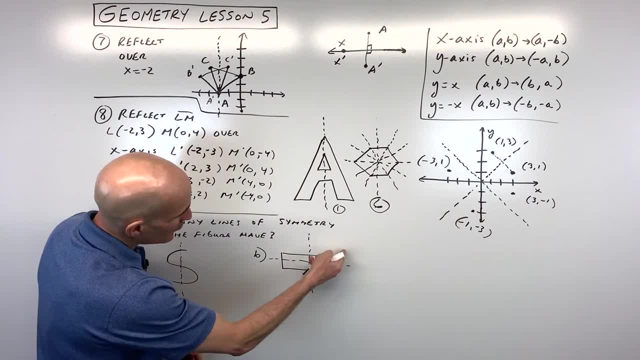 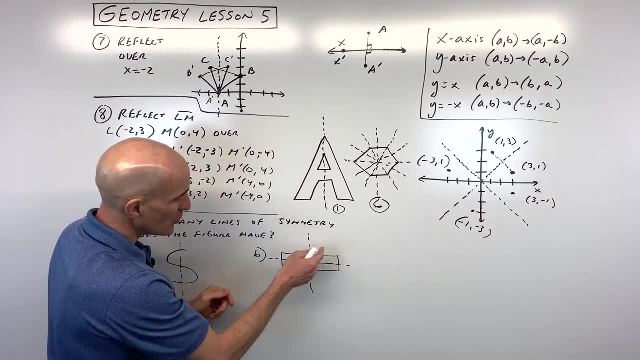 one. this way, horizontally, that would be two. how about if we go through the corners? well no, if I fold that like on a diagonal, this point's going to end up somewhere over here. this point's going to end up somewhere over here. so it looks like there's just two. 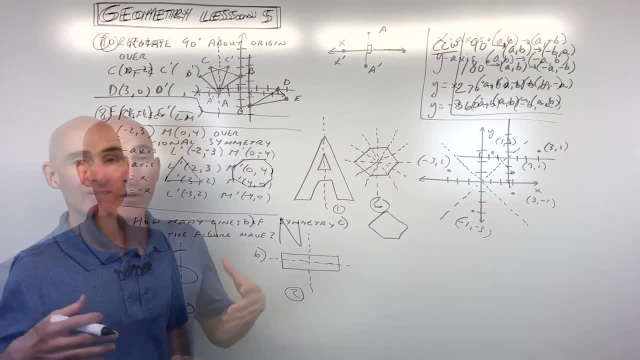 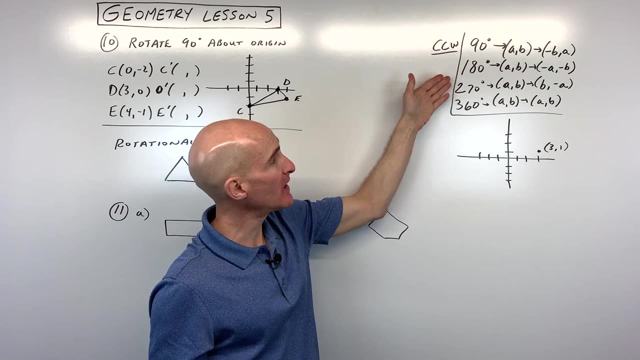 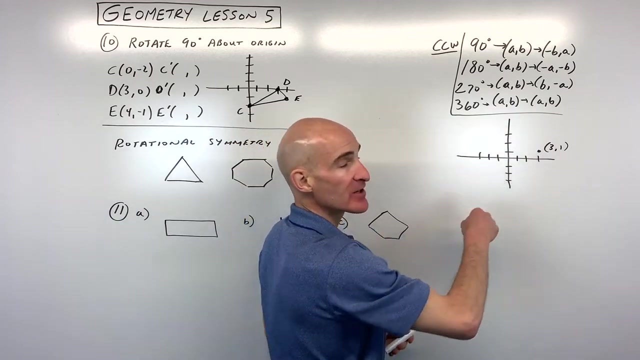 lines of symmetry. Let's talk about rotations next. okay, let's talk about rotations now. so we've got some more formulas over here, rotating 90 degrees about the origin, 180 degrees, 270, and 360, and keep in mind that these are when you're rotating counterclockwise. okay, so the opposite. 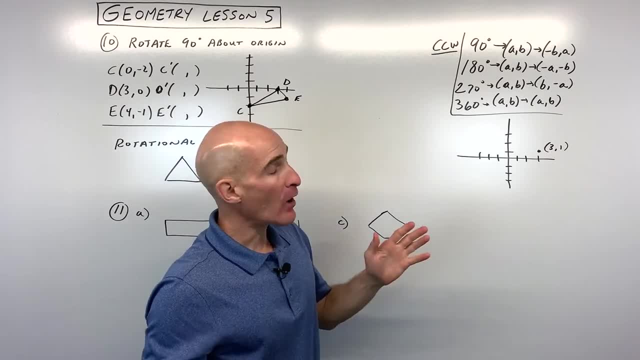 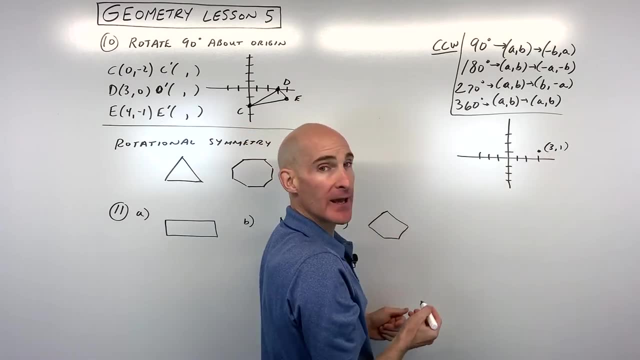 direction that the hands on a clock move. Now I want to show you how to figure this out. in case you forget these formulas, you can figure them out fairly quickly. Let's take this point three, one again. What we can do is we can make like a triangle. see if I make this into like a triangle, like 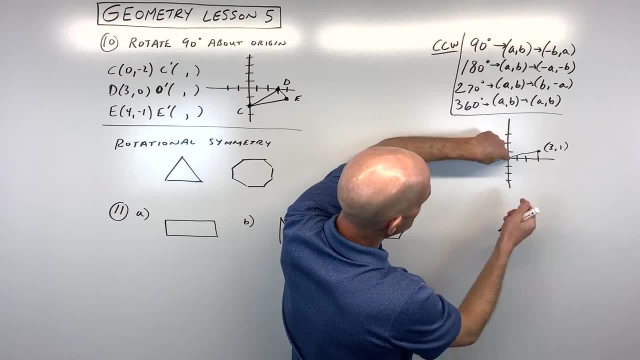 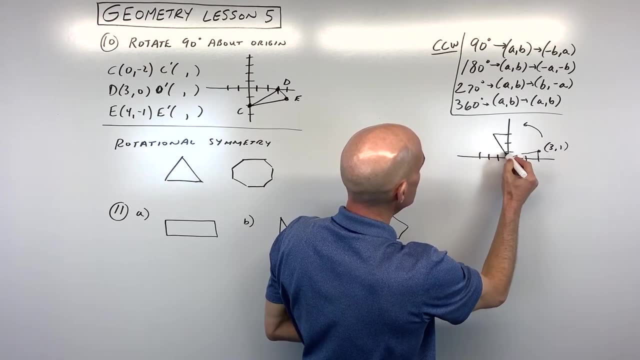 that okay. now, if I were to pick this up and rotate it about the origin, like turn it 90 degrees counterclockwise, this triangle would look something like this now, don't you agree? So this point right here is really ending up where. 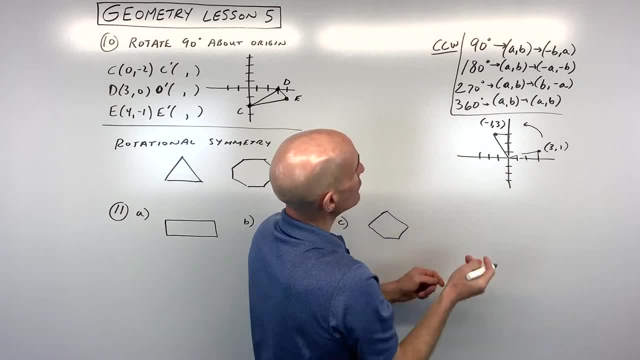 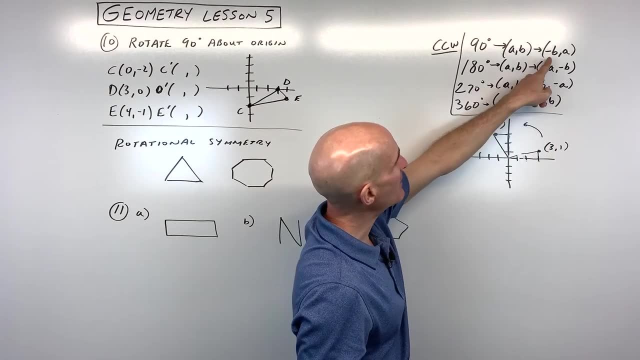 It's at negative one, positive three. and so look what happens when we rotate 90 degrees: we switch the x and the y. okay, so instead of three one, I have one, I have two and I have one three, and I make that new x coordinate the opposite sign. okay, so you're switching. 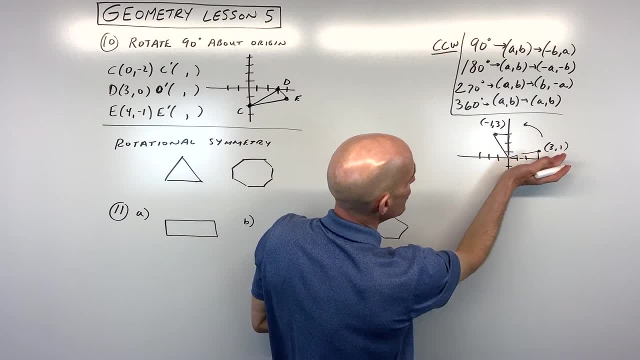 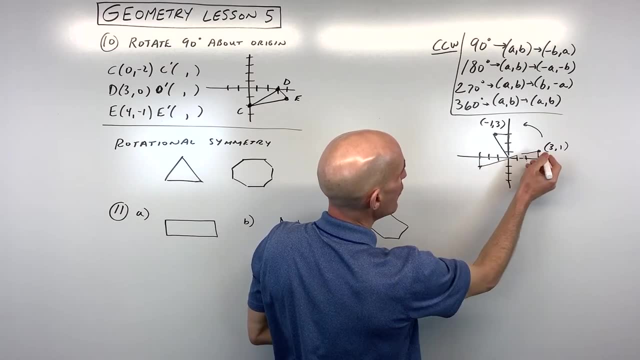 and you're making the new x the opposite. Now, if I keep going, let's say I do 180, this would be like 90, 180, you can see this triangle is going to look something like this now, and there's our point. so it's basically like: 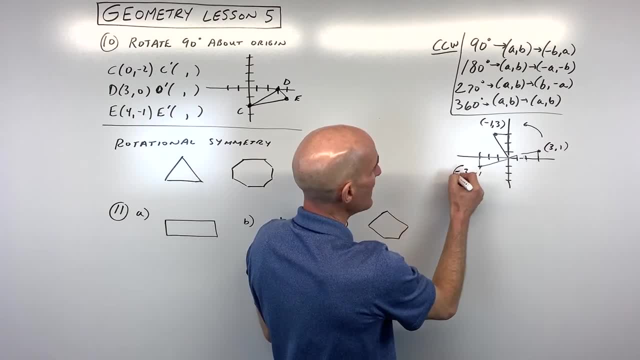 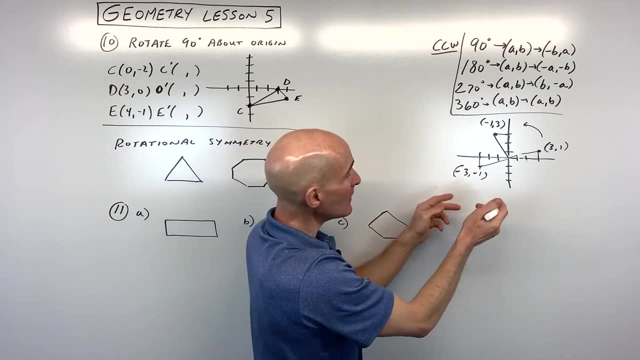 a half a turn and this coordinate now is going to be negative three, negative one. so look at what happened here. I made the x and y the opposite sign, but I kept them in the same order. If I keep going, 90,, 180, 270, now you can see this triangle is going to look something. 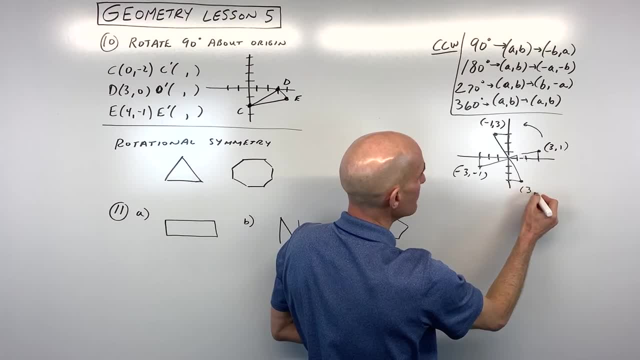 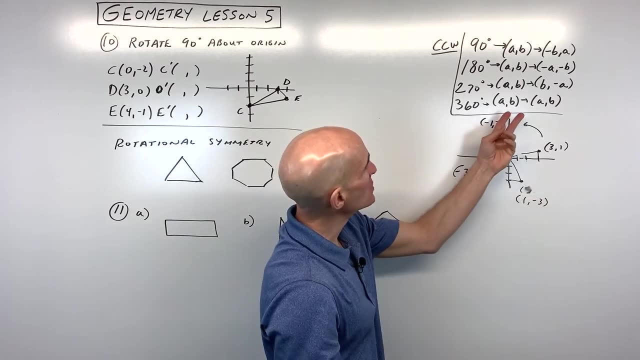 like this, and this point here is ending up at not three one, but at one negative three. so what do we do there? We switch the x and the y. we made the new y coordinate the opposite right, so I switched. 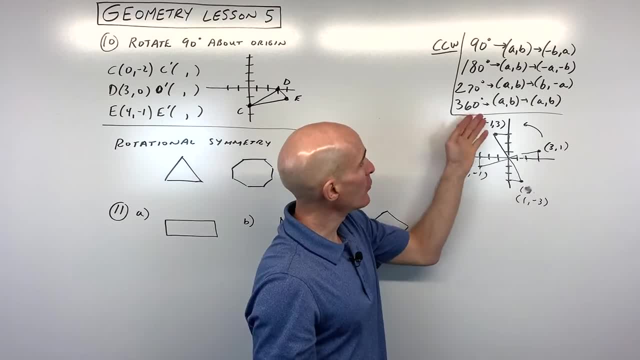 them and I made this one the opposite. So those are your rules and, of course, if you go 360 degrees- that's one full revolution- you're going to end up back where you started. so ab stays, ab three one would be three one. 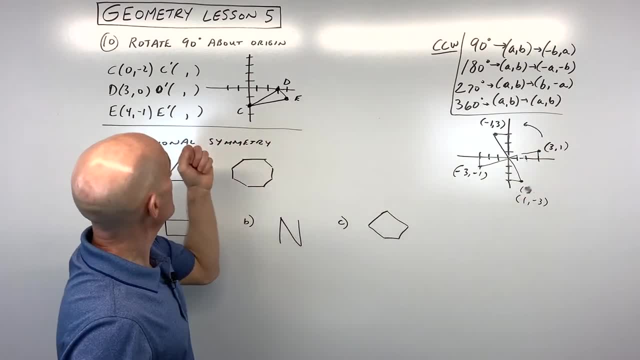 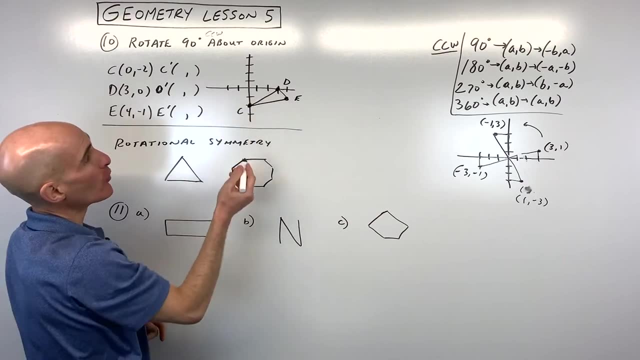 okay, so that's one full revolution. So let's go ahead and jump into some examples. say, we want to rotate this triangle 90 degrees, and I should say counterclockwise about the origin. so around this point, here we're going. 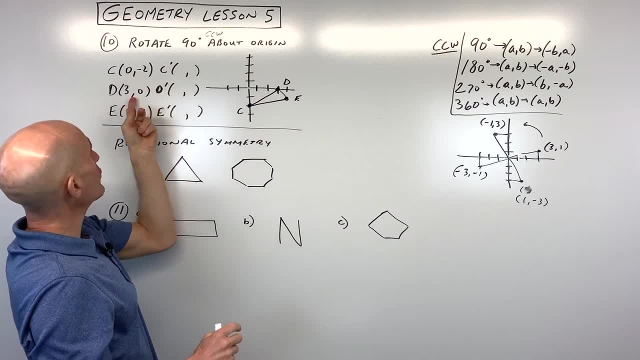 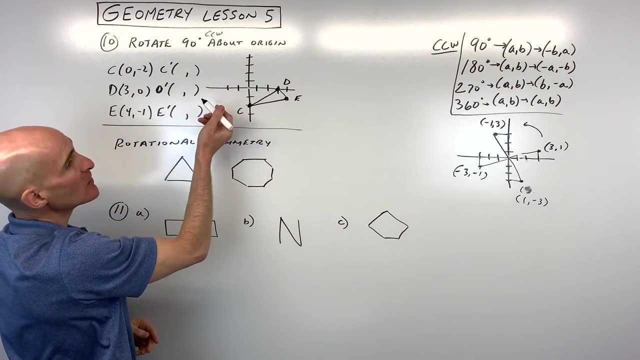 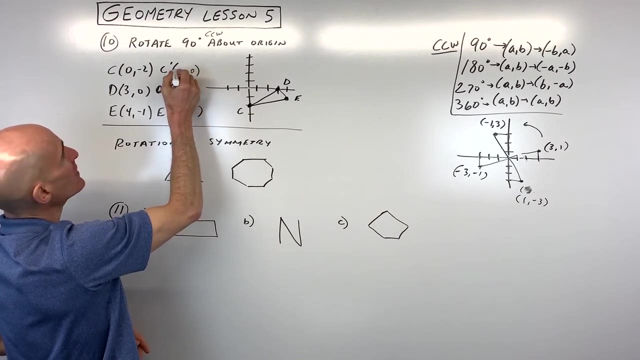 to rotate it a quarter turn. So we've got our coordinates for c, d and e, but let's use the rules now. so 90 degrees ab becomes negative ba. so what am I doing? I'm switching the order, okay, so negative two, zero. and I'm making the new x coordinate. 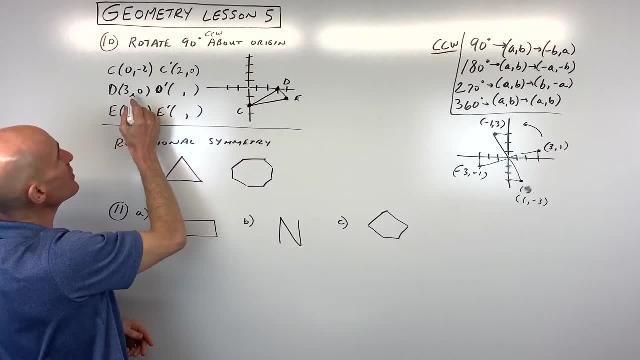 the opposite. This becomes two: zero. Same thing. here I'm going to switch these, make the new x coordinate the opposite. so this is zero. three, of course, the opposite of zero is still zero. and then same thing. here we're switching the x and y, making that new x coordinate the opposite. 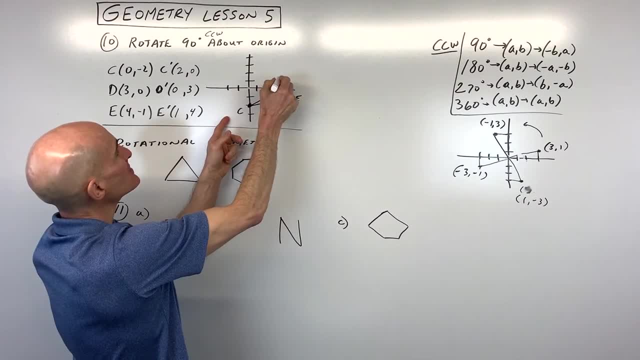 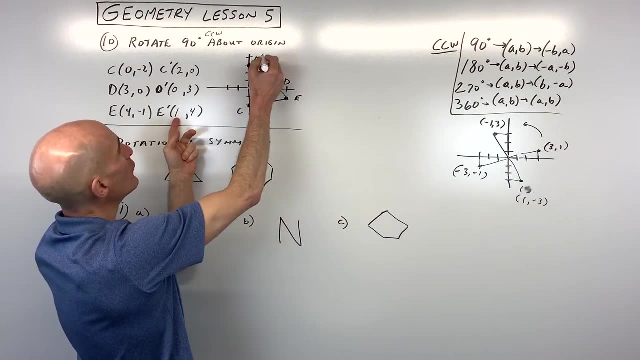 So let's go ahead and plot those now. so two zero would go here. this is c prime. d prime is zero three, that's right there. d prime and e prime is one four, which is right there. 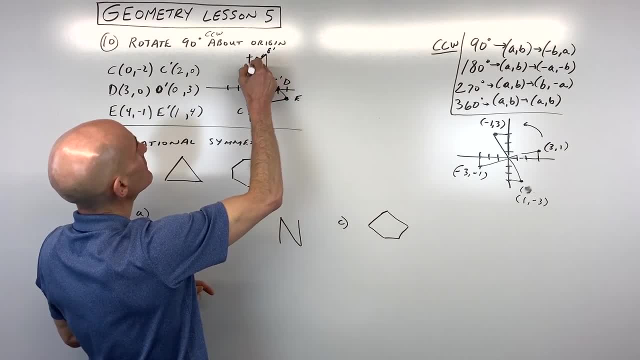 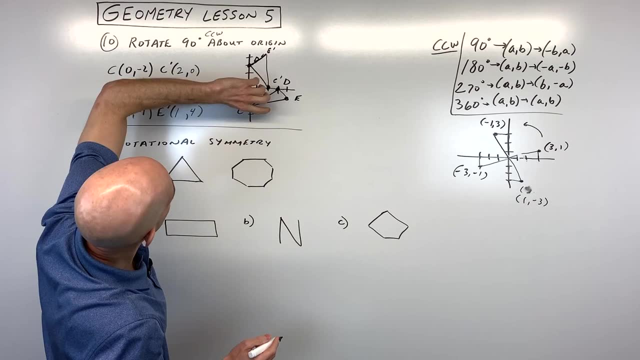 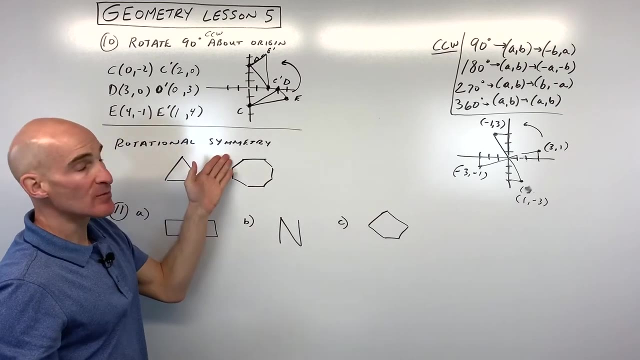 e prime. So let's see if we can connect those up. So what do you think? does that look like? it's a 90 degree rotation. We're turning it about the origin like that. okay, it looks pretty good. All right, let's look at rotational symmetry now. so, given an object, let's say we're given. 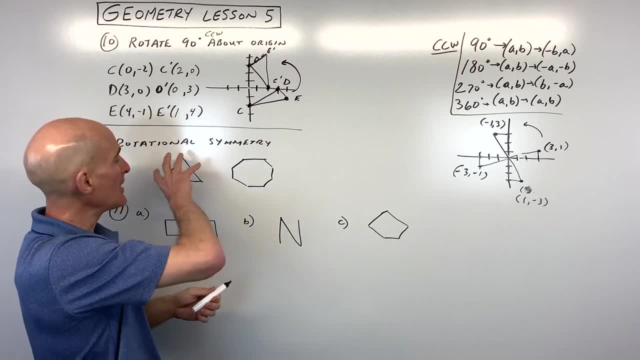 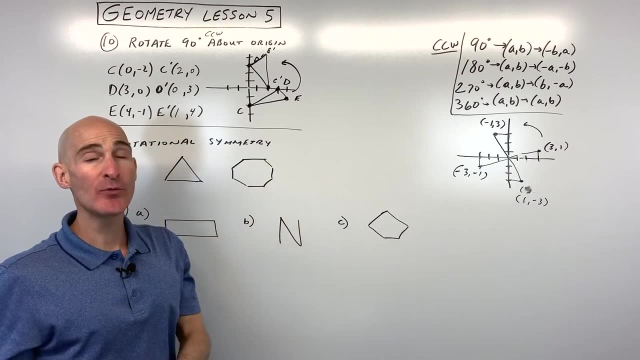 let's say a triangle or an octagon. how do we figure out how many degrees we can rotate it so that it matches up with itself? Well, there's a little bit of a trick that you can use that can sometimes help you with this. 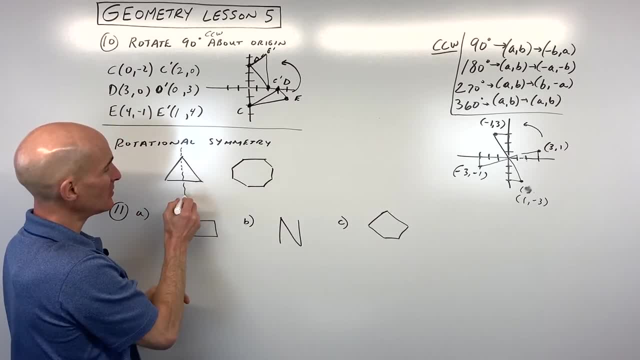 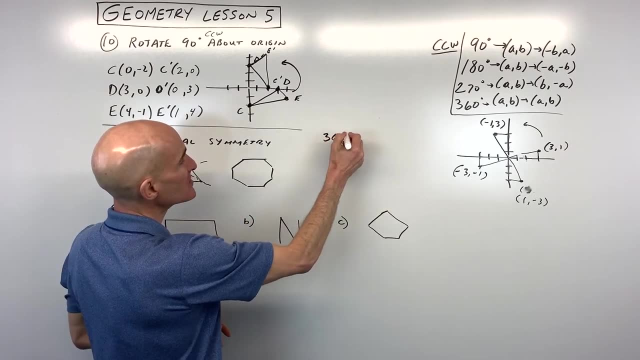 And that is revert back to finding the lines of symmetry. okay, see how there's one there, one there and one there. so there's three lines of symmetry, and if you just take 360 degrees divided by the number of lines of symmetry- in this case three- that comes out. 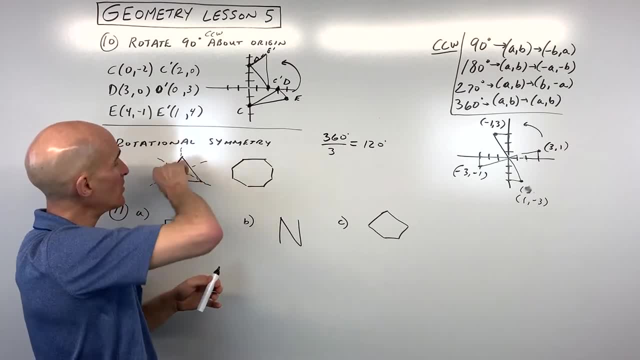 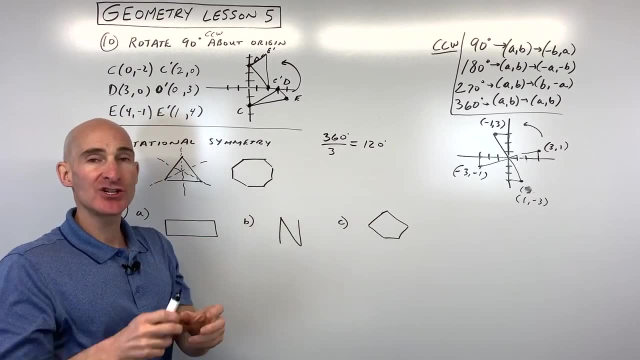 to 120 degrees. What this means is, if we rotate this 120 degrees about this point here, it's going to match up to itself. Now, when we talk about angles of rotation, we usually talk about just between zero and 180 degrees. 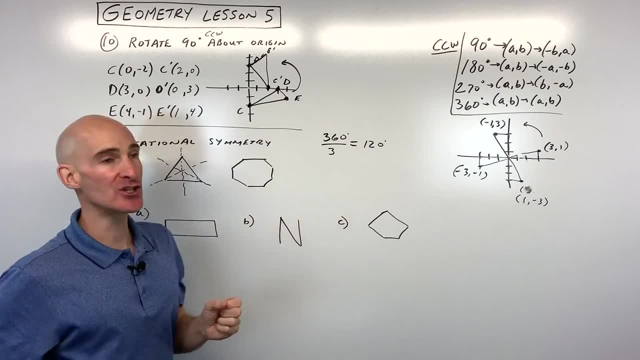 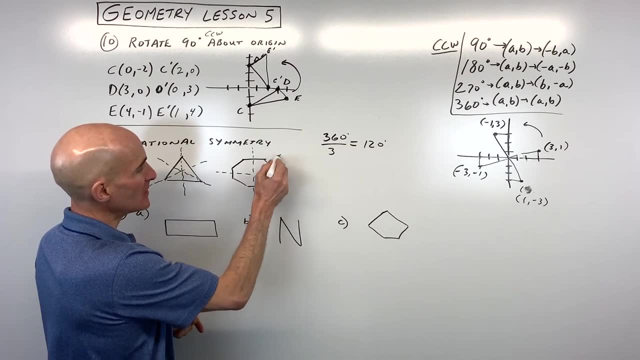 So we would just say this has to match up to itself. This has a 120 degree angle of rotation to match to itself. But let's look at this octagon. so with an octagon we can actually draw eight lines of symmetry. okay, and you can practice doing this also through the oops. I missed this. 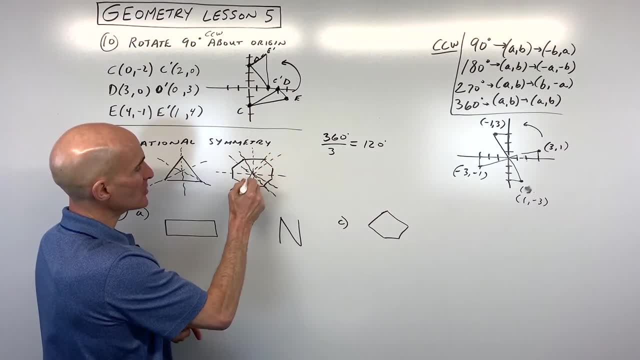 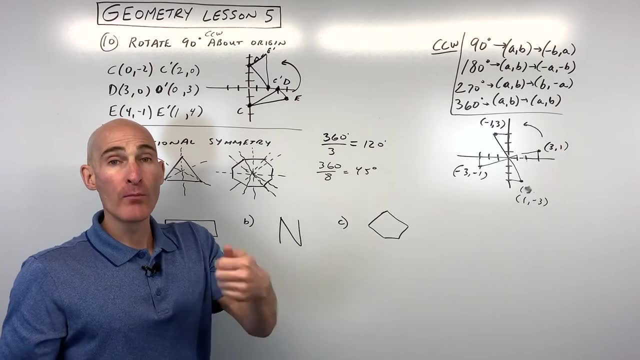 one through the vertices as well. okay, there's going to be eight of them, okay. So here, if we take 360 divided by eight, that comes out to 45 degrees, or multiples of 45, so we could do 45 times 1,, 45 times 2,, 45 times 3,, 45 times 4,, 45 times 5,, 45 times. 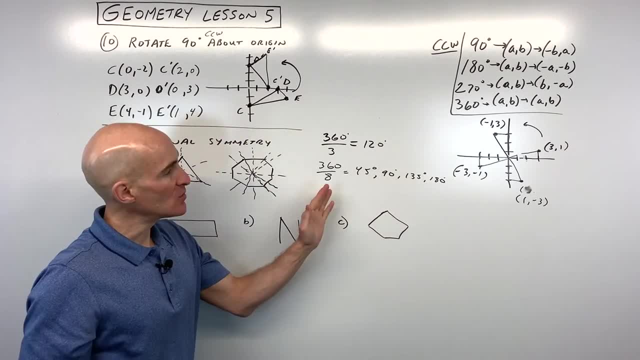 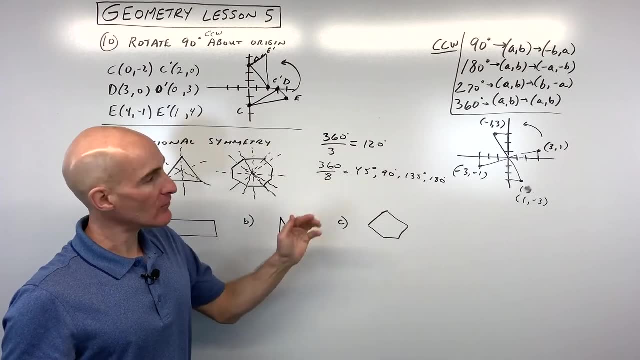 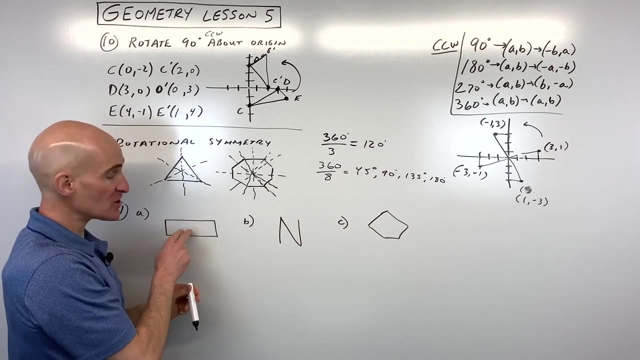 4, but we usually stop at 180, so we just say the angles of rotation up to 180 would be these angles of rotation. We wouldn't keep going forever and ever just between zero and 180.. So see if you can do that for number 11. here A, B and C, what's the angle of rotation? 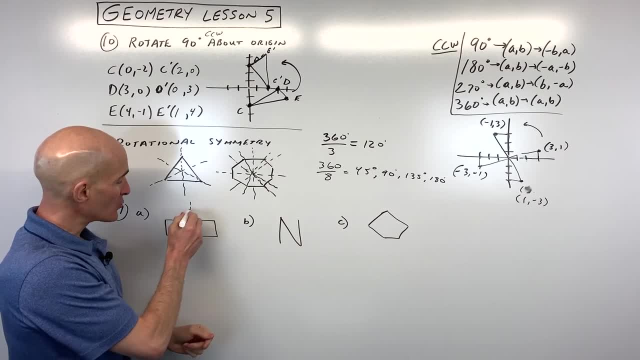 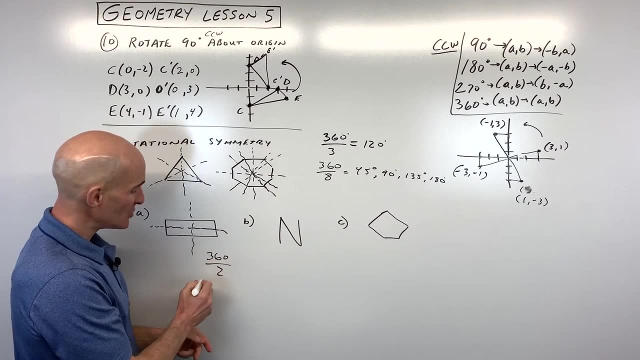 for this figure here. Well, you might say: okay, Mario, I know I can draw a line of reflection there, a line of reflection there. that's two lines of reflection. so 360 divided by two is 180 degrees, right? Yep, that's exactly right. you could turn it a half turn and it's going to match up. 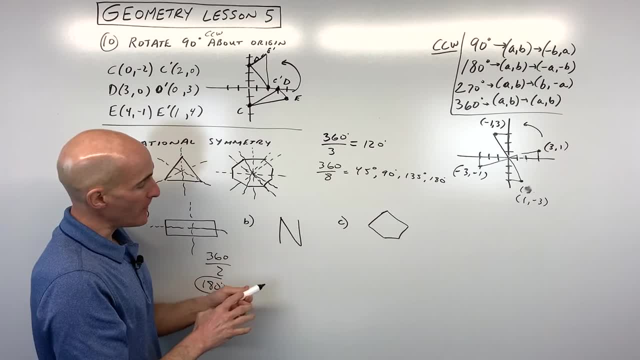 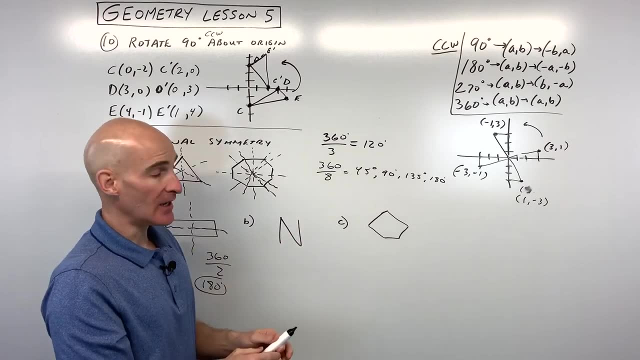 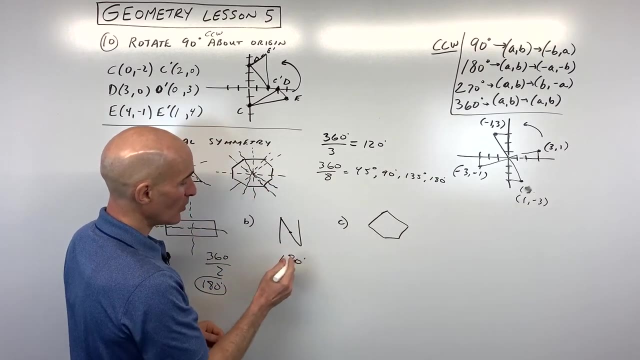 with itself. For letter B, what do you think for this one? How many degrees do we need to rotate this? Well, you're probably realizing that there's no lines of symmetry here. okay, but you can still rotate it. See, if I take this point right here and if I turn this a half turn, 180 degrees, it will. 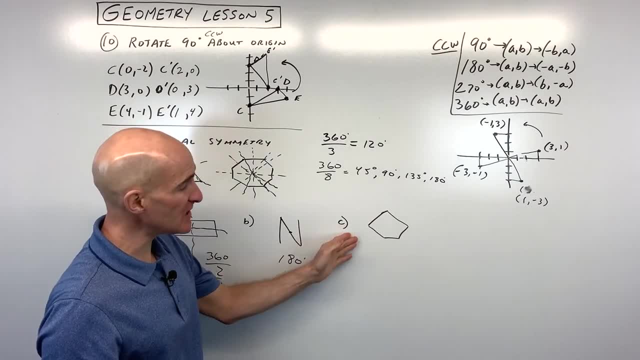 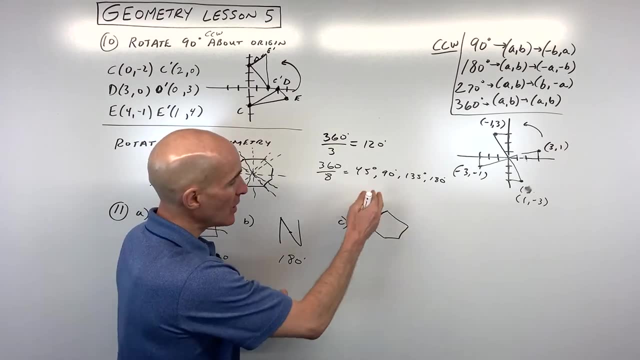 match up with itself. so 180 degrees. and for letter C? what do you think for that one? Well, here, because it's a pentagon, okay, and a regular pentagon. All the angles are the same, all the sides are the same. you're going to have five lines. 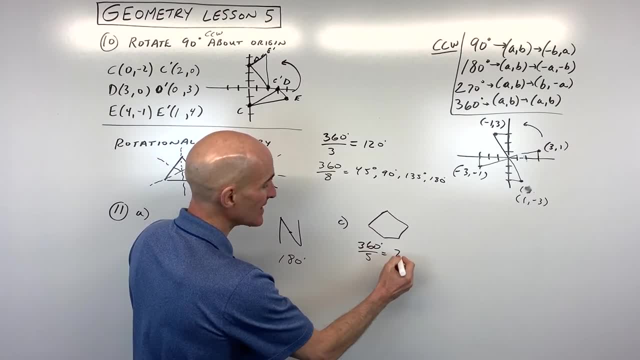 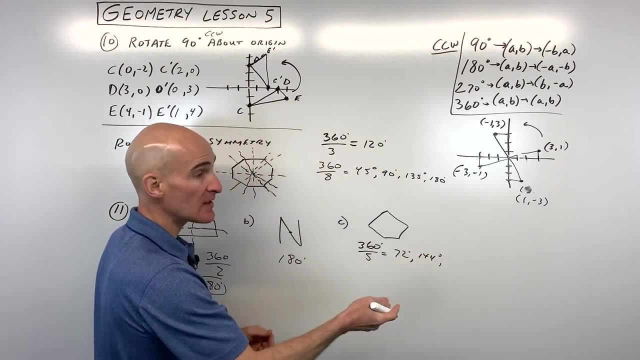 of symmetry. so 360 divided by 5 is 72 degrees, or multiples of 72, right? So 72 times 2,, that would be 144, 72 times 3,, that's going to exceed 180, so we're just. 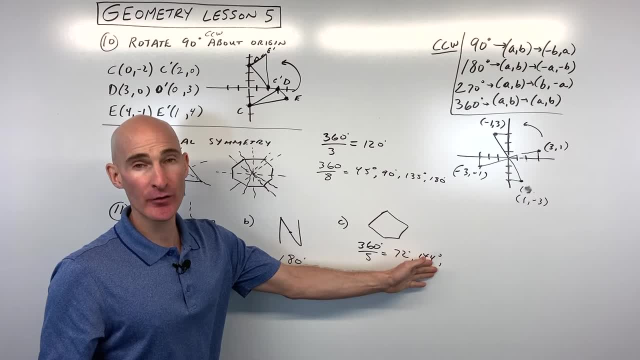 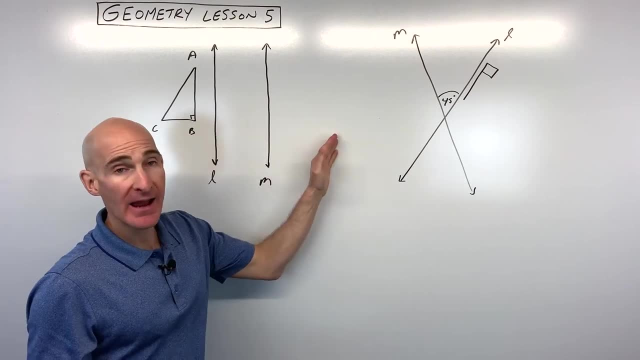 going to list the ones between 0 and 180, 72 degrees and 144 degrees. Okay, before we get into dilations, I want to show you what happens when you reflect over parallel lines or if you reflect over intersecting lines. 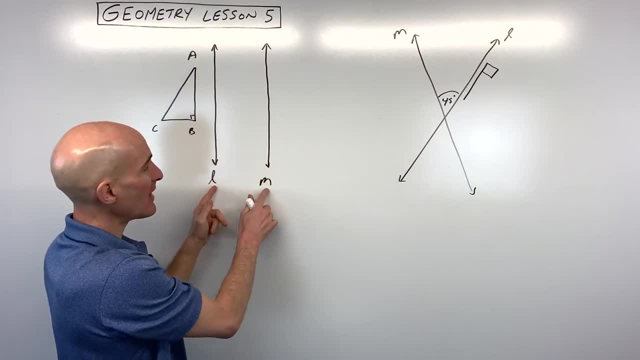 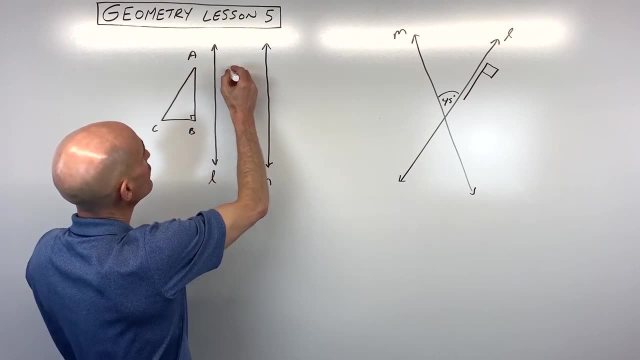 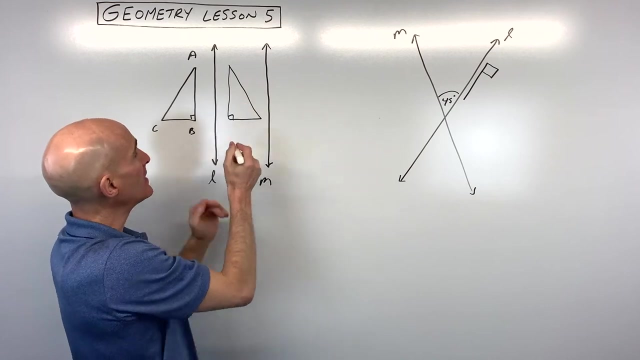 So let's start with parallel lines first. so say we have lines L and M, they're parallel, they don't cross. let's say we take this triangle first, we reflect it over line L. so remember if we do that it's the same distance from the line, okay, perpendicular to the line. 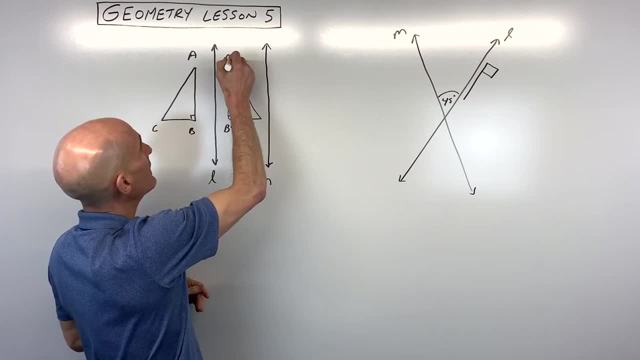 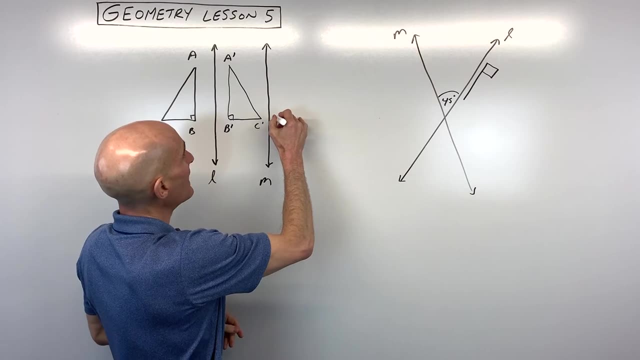 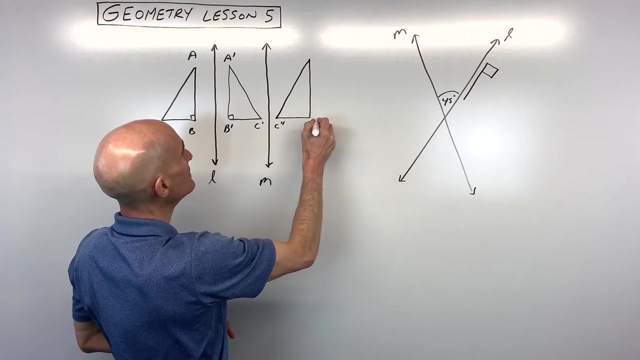 so this should be B prime, A prime and C prime. Now let's go ahead and take that image, reflect it again over line M. we should get a triangle that looks like this: okay, so now we have C double prime, B double prime. 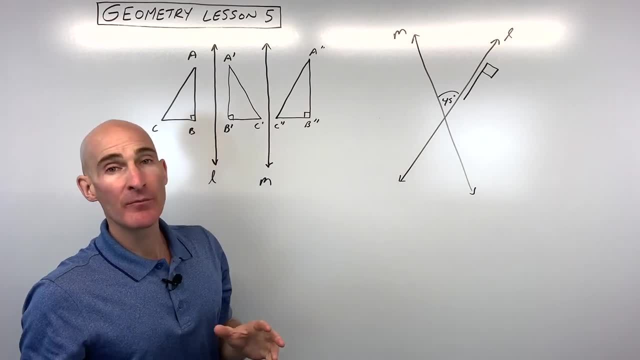 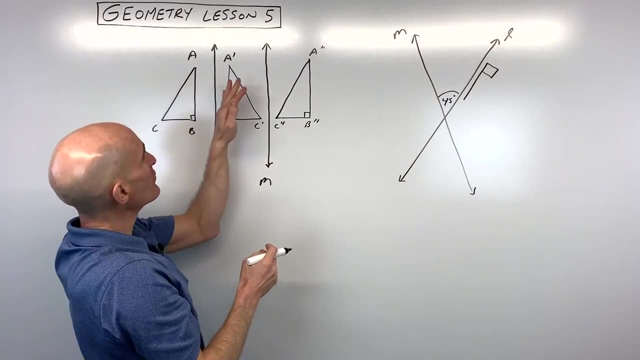 and A double prime. But what I want to show you is that what happens to this original figure, this pre-image here, all the way to the final figure? well, see, when you first, when you reflect it, see how it's kind of. this is kind of pointing to the left, now it's like pointing to the right. 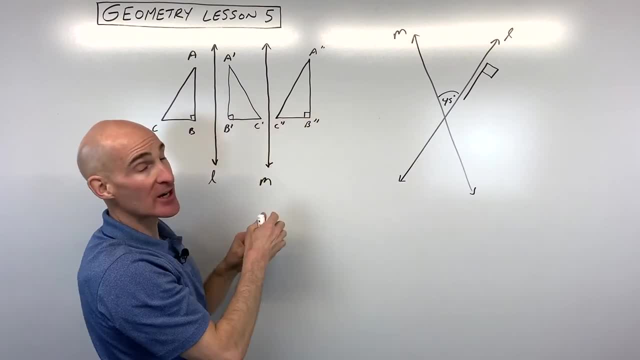 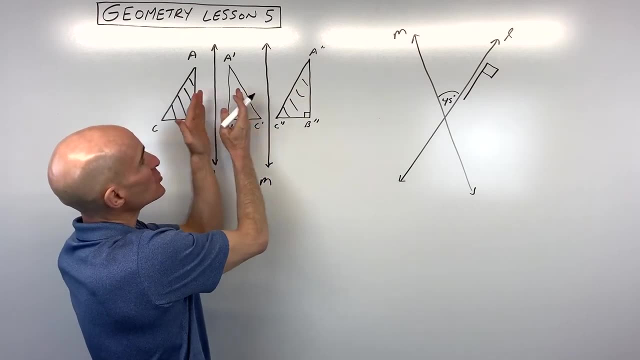 but when we reflect it again, then see how it's kind of like pointing back the original direction. So what we did is, when we did that double reflection over the parallel lines we're going to see it ended up being a translation, a slide, a shift, right. 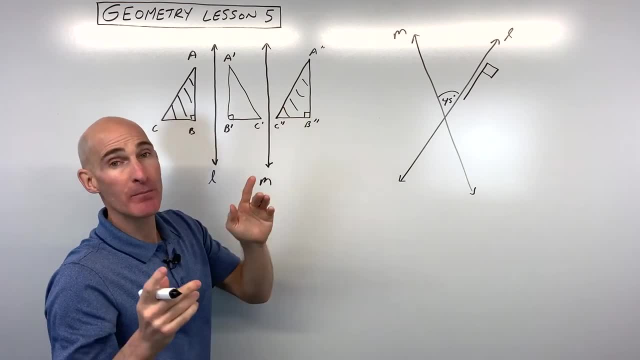 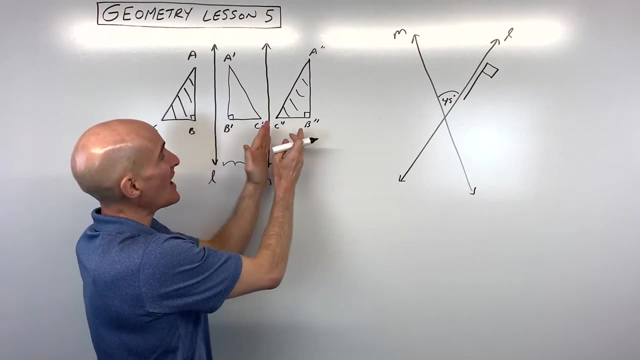 So that's the key is when you reflect over parallel lines. it's a translation, but it's double the distance between the parallel lines. so say this is one inch, okay, it would actually slide two inches. or if this was, you know, one foot, this would slide two feet okay. 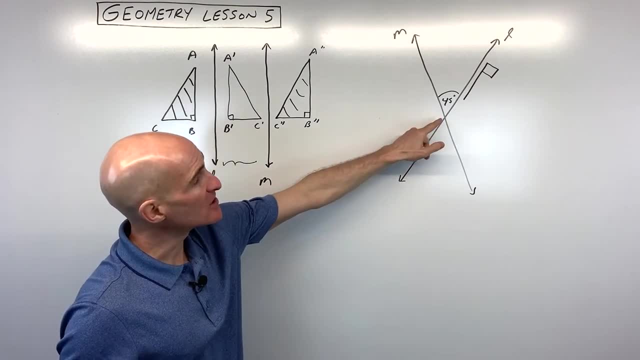 it's going to be double, And so that's the key there. Now, when the lines are intersecting, what you want to do if we reflect over line L and then we reflect over line M? let's look at what that looks like. 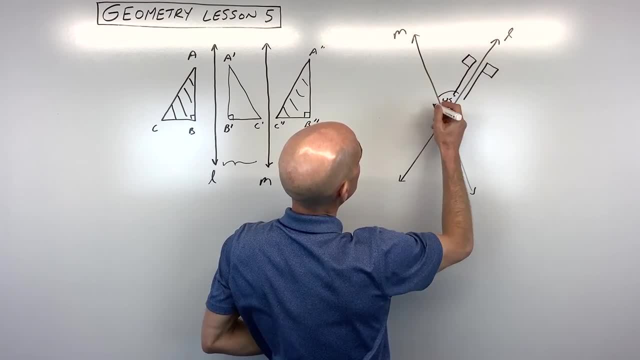 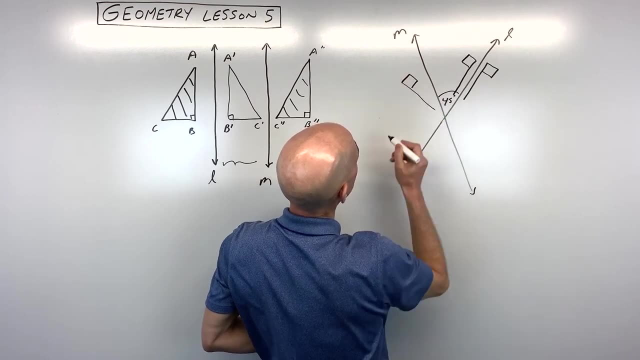 So it'd look like a flag facing this way, and then, if we reflect over here, it looks like it would be a flag facing. let's see, what would this be like? something like this: Okay, not perfect, but you're reflecting over like that. 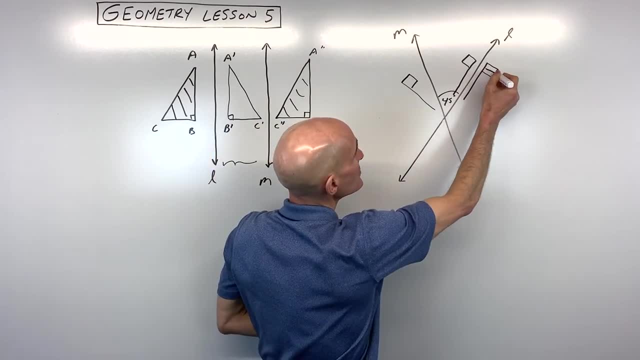 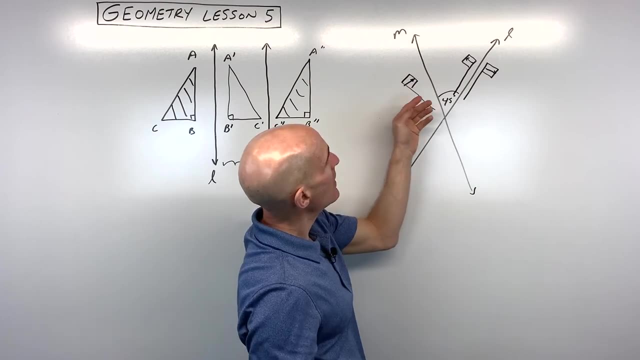 Now what happens is again, let's just draw an arrow so see how it's pointing to the right. now it's pointing to the left. okay, now we reflect it, it's pointing back to the. you know this other direction. 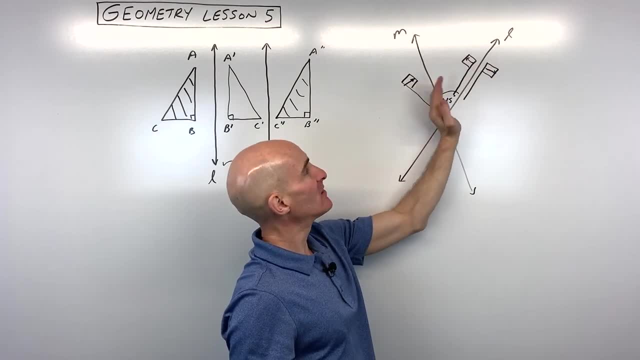 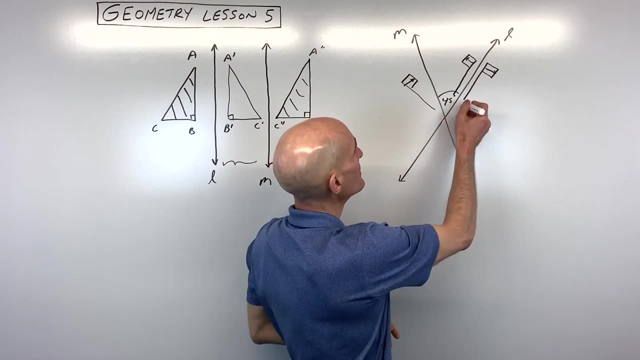 But it actually ends up being a rotation. okay, so from this original figure it's going here to the final figure. here we did a reflection, reflection, but the final result from here to here is a rotation. double that angle between the two intersecting lines. 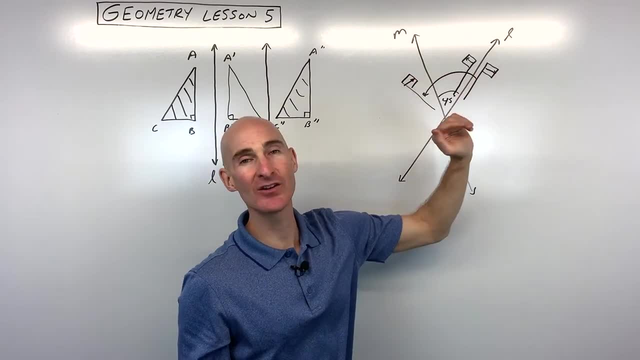 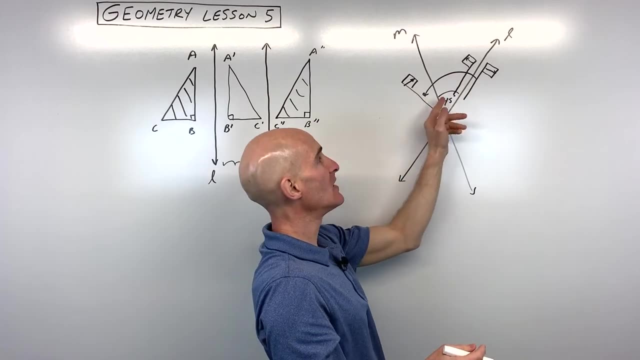 So if this is 45, you can see that it actually rotated double 90 degrees. So here it's translating double the distance, okay, between the parallel lines. here it's rotating double the angle between the intersecting lines, Okay. the final type of transformation that we're going to talk about are dilations, and 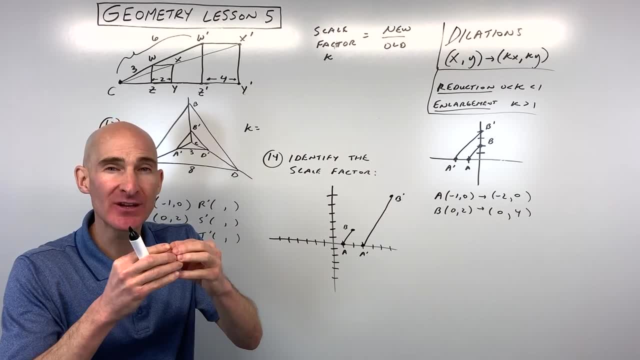 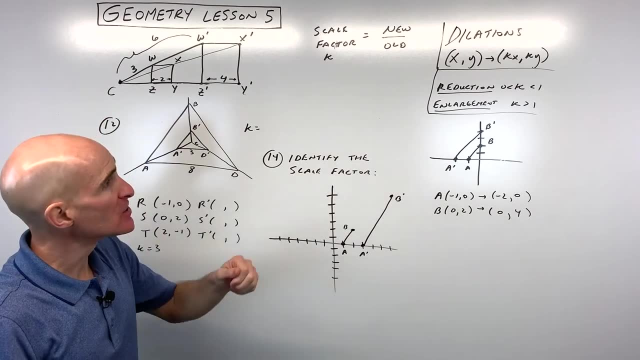 what exactly is a dilation? Well, dilation is okay. what is a dilation? A dilation means that it's either getting like larger, like it's expanding, or it's like a reduction, it's like shrinking, it's getting smaller. 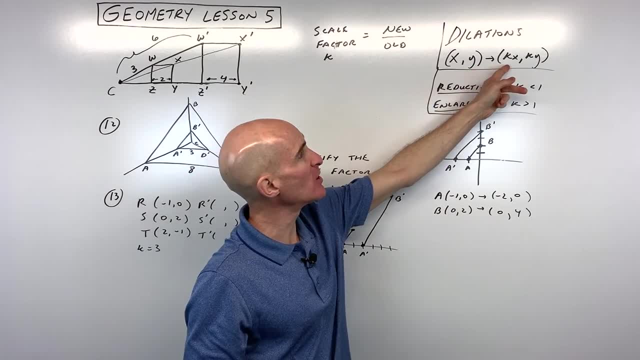 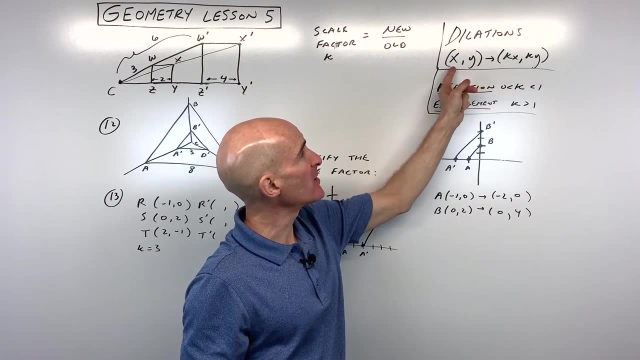 So when we talk about dilations, we have one formula here that we're going to be using when you dilate or expand or contract towards the origin or from the origin, and it's this formula here: xy maps to k times, x, k times y. 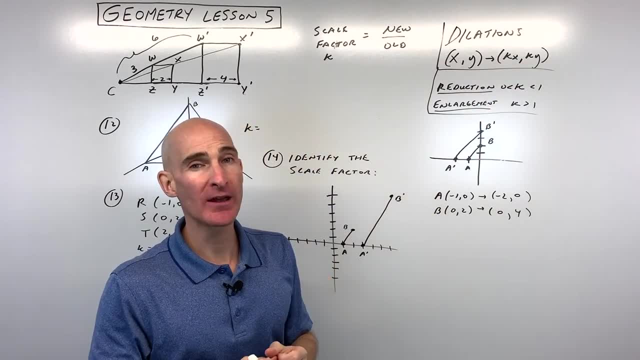 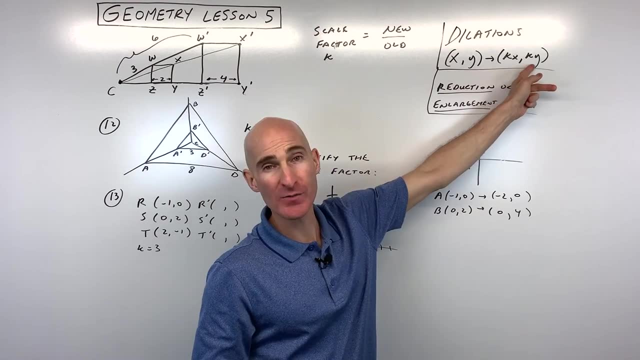 Now, what's k? Well, k represents the scale factor. so, like if you were doubling- you know, making it like double- you would multiply the x's by 2 and the y coordinates by 2, and that's going to be, like you know, an enlargement by a scale factor of 2.. 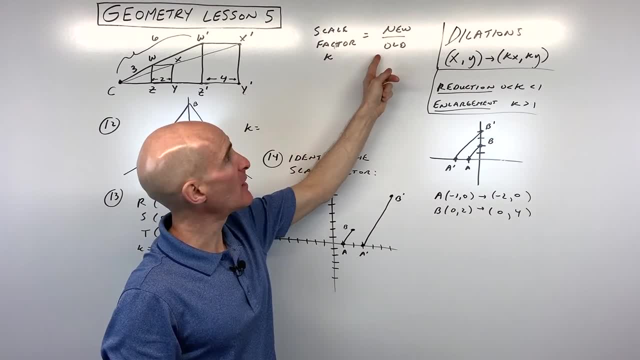 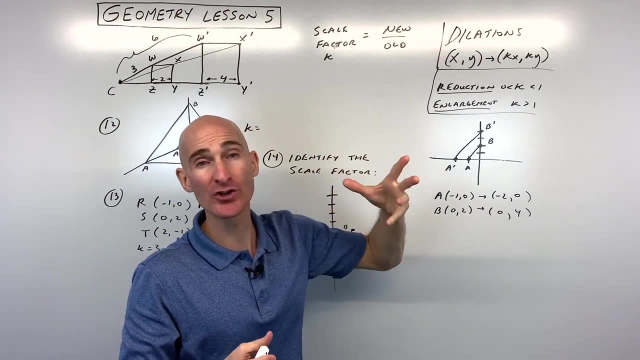 Another way you can look at the scale factor is you can look at the new figure divided by the old figure. So if you compare, like the side lengths of the new figure and old figure, if you take the new side length divided by the old side length, the original one, that'll give you 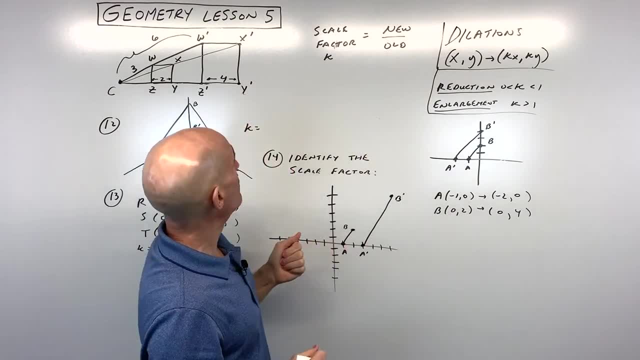 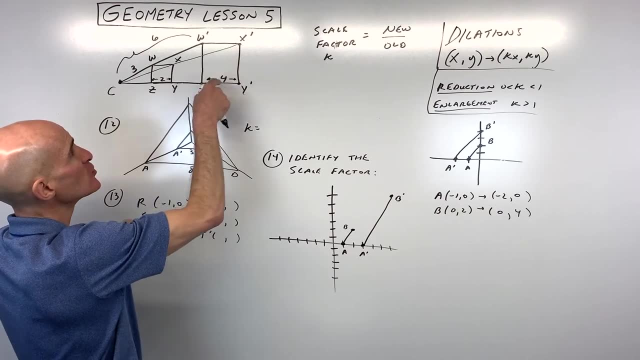 your scale factor. So just remember new over old. Now let's just take a look at this one over here Say: we have like a square, This is like our preimage And this is our image. This is the new square. So it's kind of like if you take like a flashlight, you're shining it at the square and it's projecting. 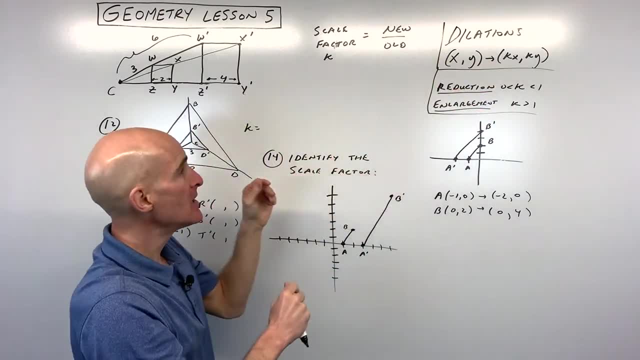 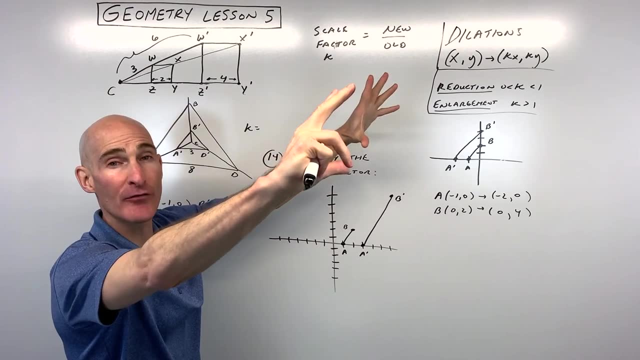 that new square up on the wall. So you can kind of visualize that, This point where the flashlight is projecting from, that's what's called our center of dilation. It's where everything is expanding out from or, you know, reducing or contracting back. 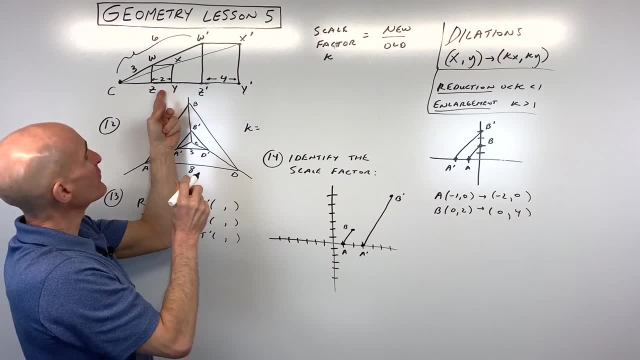 towards. okay. So what we can do is we have two options here. when we're figuring out the scale factor, We can either look at: okay, here's the new length of this square. I'm sorry, here's the old length, here's the new length. 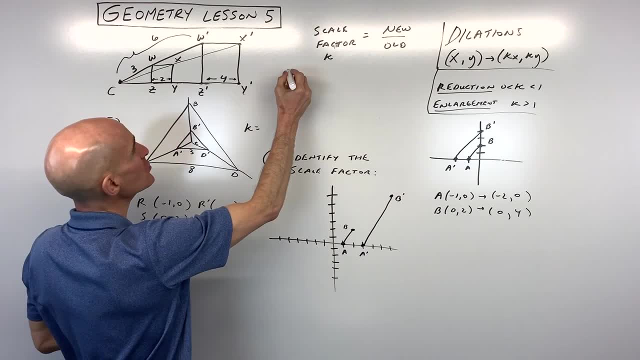 We take the new length, which is 4, divided by the old length, which is 2.. So 4 divided by 2 gives us the scale factor of 2.. So this is an enlargement with a scale factor of 2.. 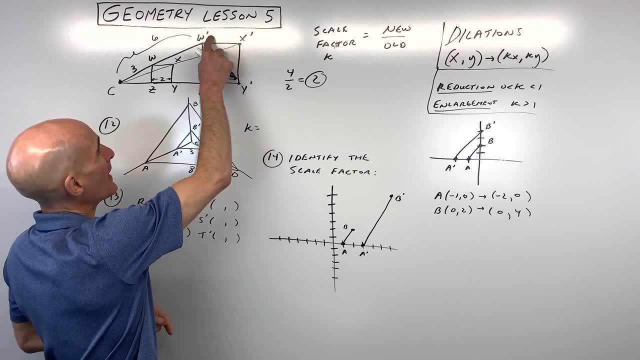 Now, how did I know this was the new one? Well, I knew it was the new one because I see the primes. The prime tells us it's the new one. Without the prime, that's the old one. right, That's the preimage. 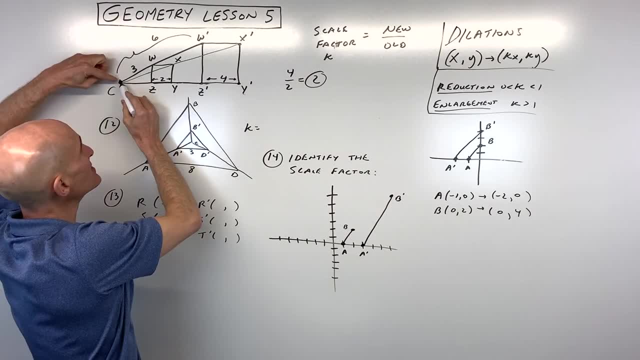 This is the image. The other way to do it is: you can measure the distance from the center of dilation. So I could say: well, from C to W- prime, that's 6.. From C to W, that's 3.. 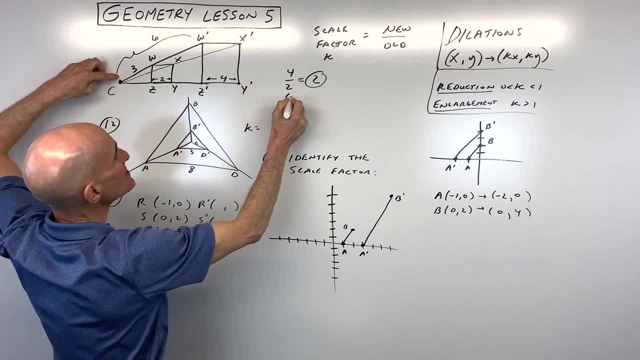 That's 3.. So I'm taking that new length from the center of dilation, which is 6, divided by the old length from the center of dilation, that's 3.. 6 divided by 3 also gives us 2.. 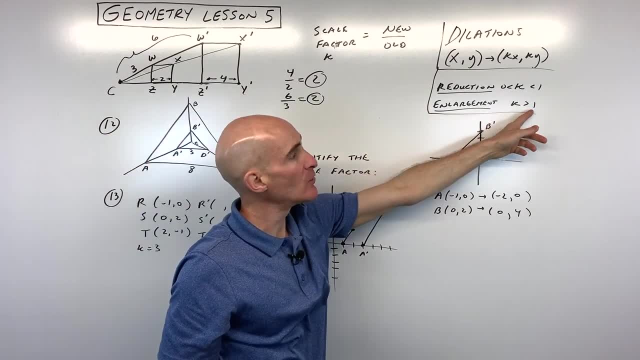 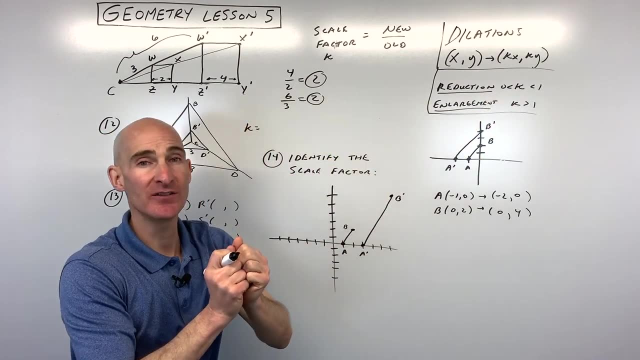 So that's the scale factor of 2.. Now when the scale factor is greater than 1, we call that an enlargement. When the scale factor is between 0 and 1, like a half or a third, that's a reduction. 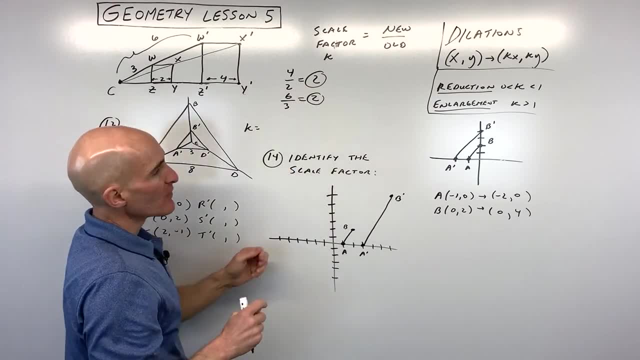 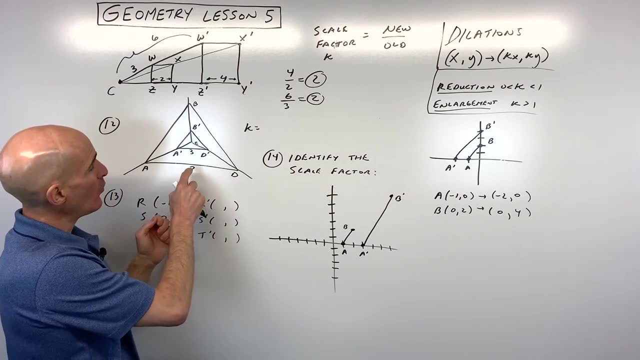 So you can tell whether it's an enlargement or a reduction by the scale factor. Let's look at this one, next, number 12.. So how would you do this one? Is this an enlargement or a reduction? Well, you're probably saying: Mario, I can see that A prime, B prime, D prime, this triangle. 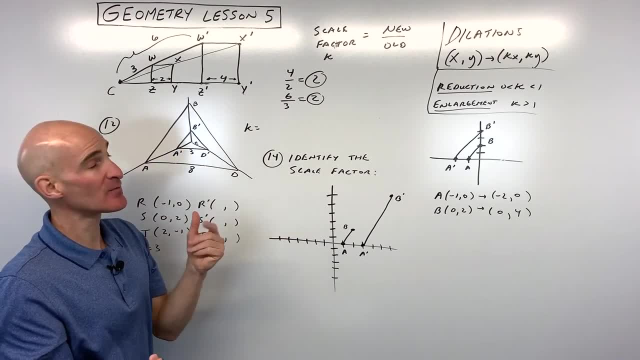 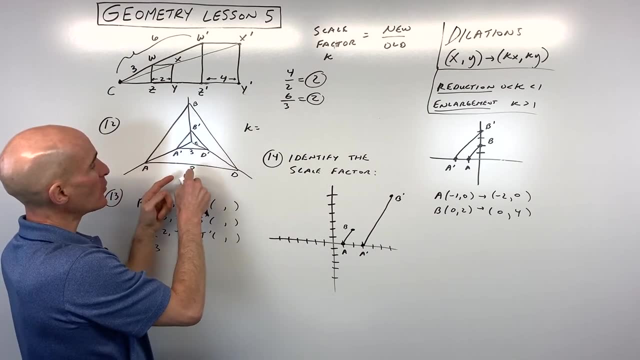 here is actually smaller. so I know it's a reduction, just because I can tell it's smaller. So you're right about that. Now to find the scale factor: see, we're going from this larger triangle to the smaller triangle. We want to take the new length, 3, divided by the old length of this triangle, here 8.. 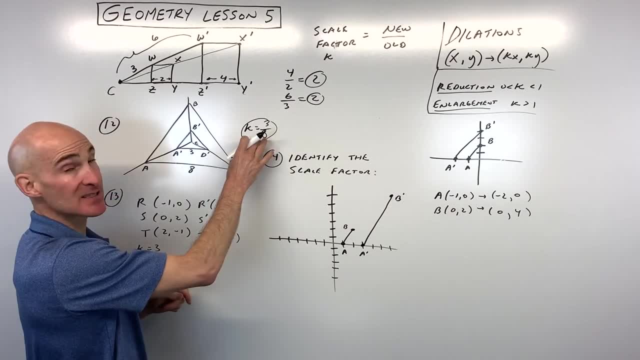 So the scale factor K is 3 eighths and we can see it's less than 1.. It's between 0 and 1.. That's a reduction. Okay, So we knew that, just because we could tell it was smaller, right. 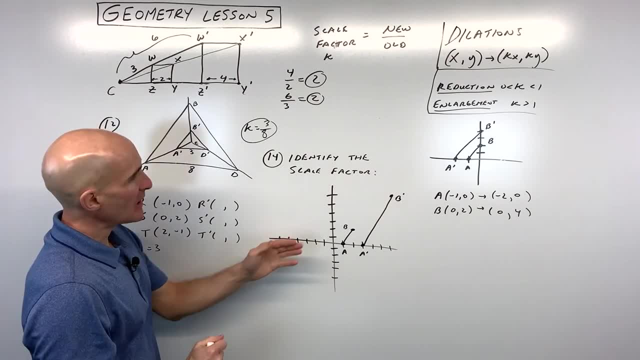 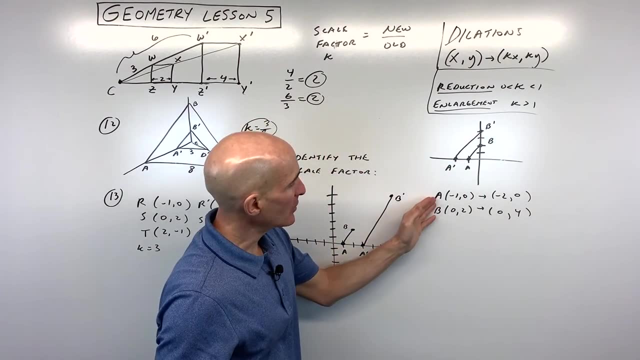 Okay for number 13,. let's look at this one actually here first. So first I want to show you, say we have this segment AB and we have the new segment A prime, B, prime. and look at the coordinates here: negative 1, 0 for A. negative 2, 0 for. 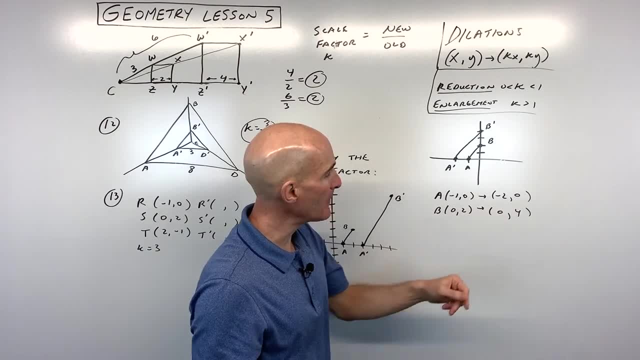 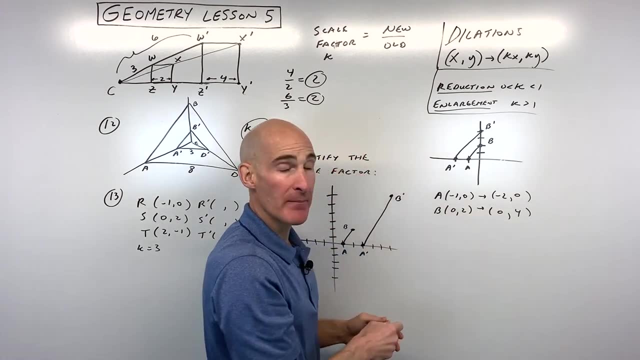 A prime: 0, 2 for B, 0, 4 for B prime. What's happening to get from this coordinate to this coordinate, this coordinate to this coordinate? Well, if you said you know you're multiplying by 2, you'd be right and you can see that. 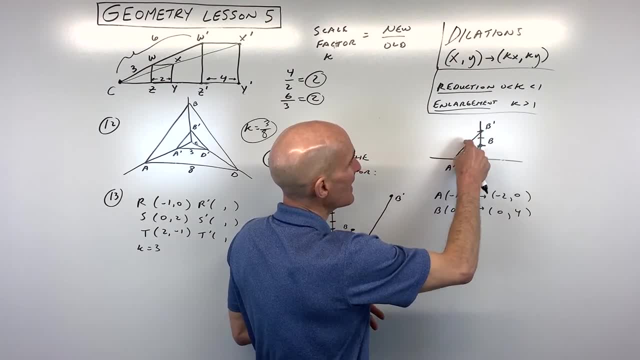 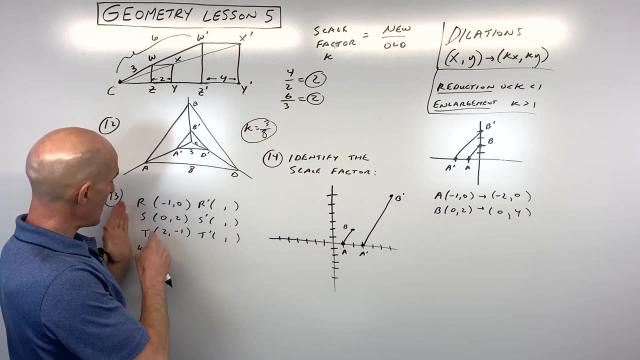 this is expanding out from the origin and you can see that that, you know, is an enlargement with a scale factor of 2.. Now let's go to number 13. now. So say you have a triangle with vertices R, S and T, but you want it to be an enlargement. 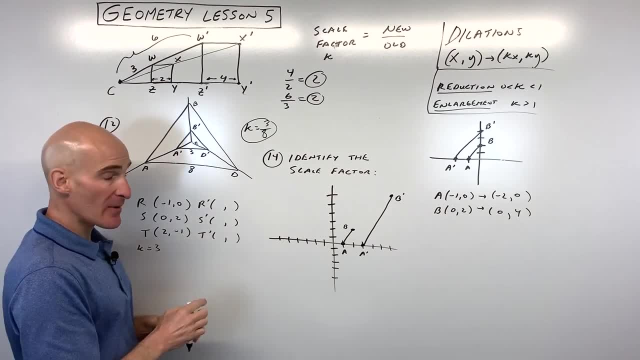 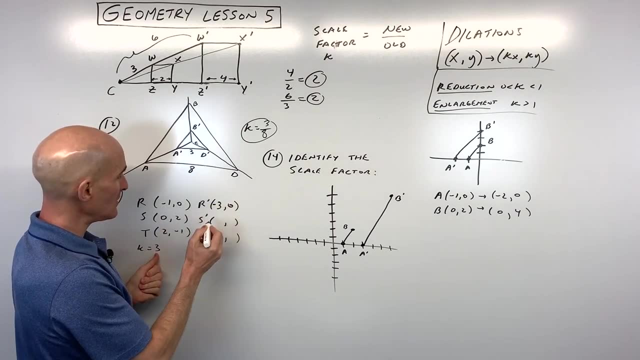 with a scale factor of 3.. So what would be the new coordinates? R prime, S prime, T prime. Well, super simple, super easy. You just have to multiply the X's and Y's both by 3.. That's negative 3.. 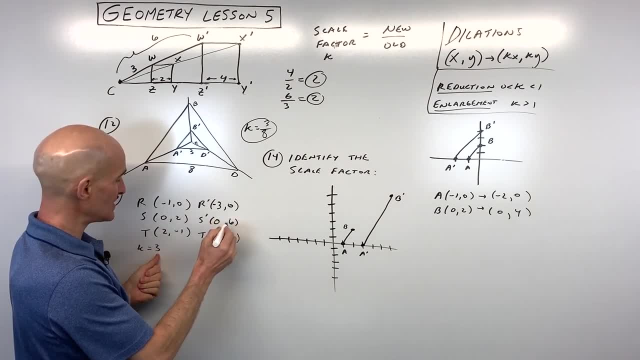 0 times 3 is 0.. 0 times 3 is 0.. 2 times 3 is 6.. 2 times 3 is 0.. 2 times 3 is 0.. 2 times 3 is 6.. 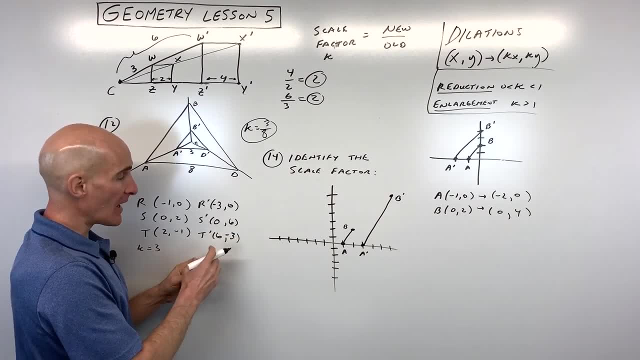 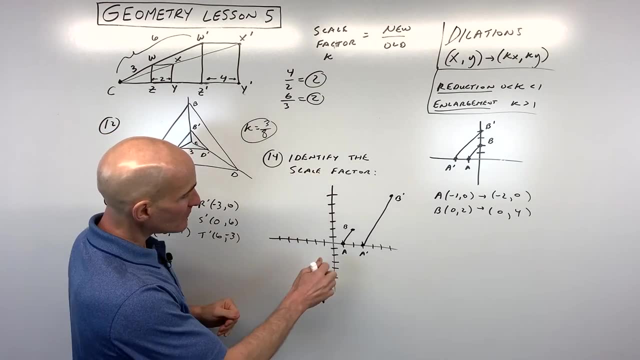 And negative. 1 times 3 is negative 3.. Now if you plot it, you'll see. you know what's happening. It's being enlarged. The last one here: identify the scale factor from this segment to this segment. You can do this a couple different ways. 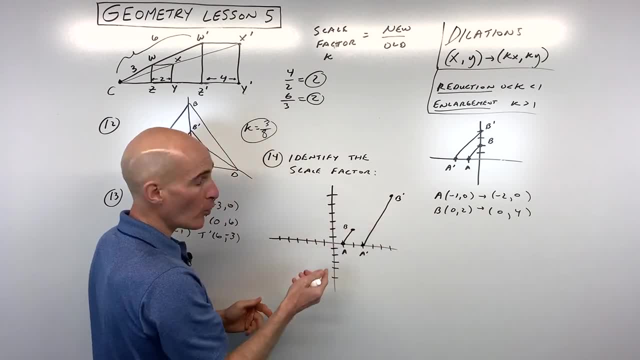 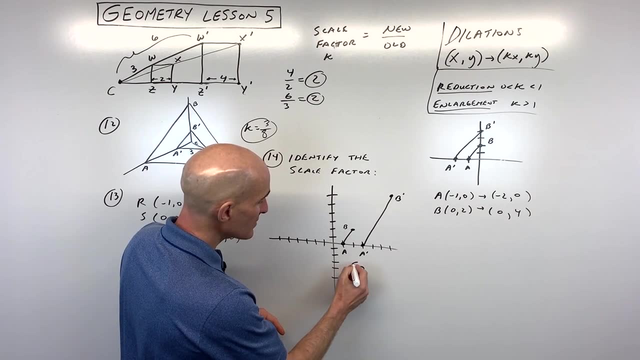 Like if I knew this length and I knew this length, I could take the new length divided by the old length. I don't have that to go on, so I'm going to look at the coordinates of the points. the endpoints A is at 1, 0. 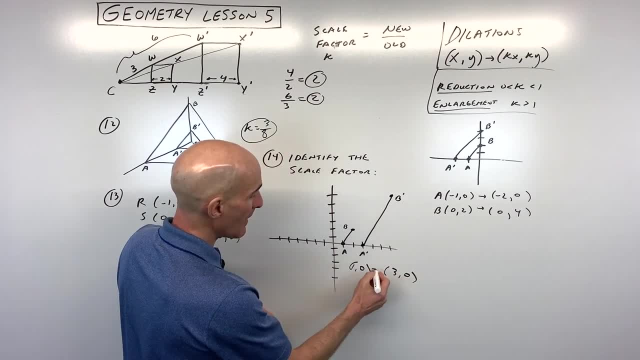 A prime is at 3, 0.. So what do you think happened there? Looks like we're multiplying by 3.. Let's confirm with the coordinate for B. here B looks like it's at 2, 2.. B prime looks like it's at 6, 6.. 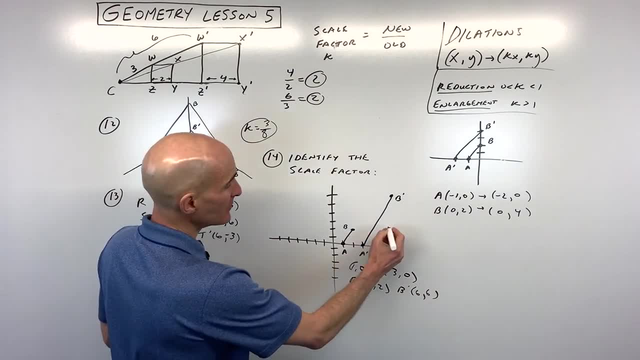 So you can see it looks like we're multiplying the X's and Y's by 3.. So this is definitely an enlargement. The scale factor is 3, and you got it.